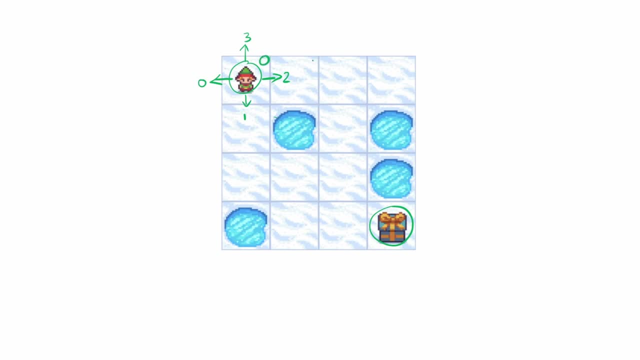 spot. Internally, we're going to represent each state, as this one is zero. this one is one, two, three, four, five, six, all the way to 14,, 15.. So 16 states total. Each attempt at navigating the. 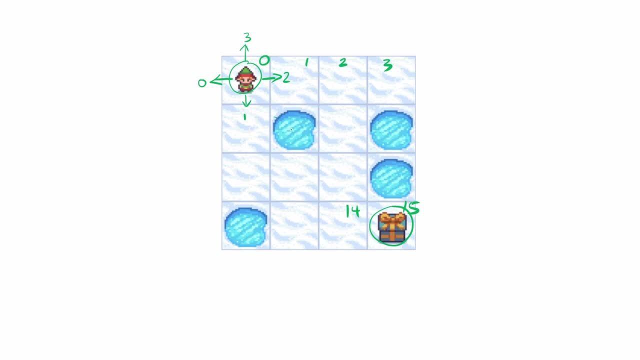 map is considered one episode. The episode ends if the agent falls into one of these holes or it reaches the goal. When it reaches the goal, it will receive a reward of one. All other states have no reward or penalty. Okay, so that's how this environment works. At this point, you might be wondering why we would need 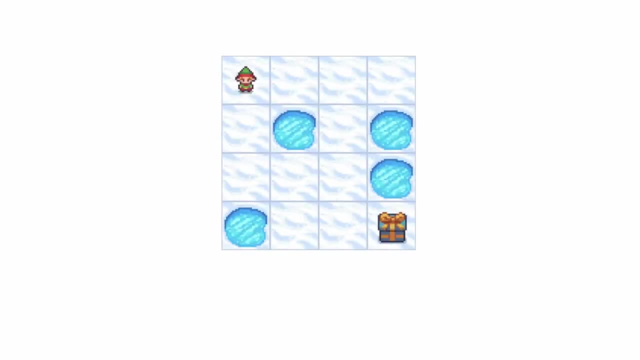 reinforcement learning. to solve such a simple map, Why not just use a pathfinding algorithm? There is a twist to this. There is a flag called isSlippery. When set to true, the agent doesn't always execute the action that it intends to. For example, if the agent wants to go right, there's only a one-third chance that. 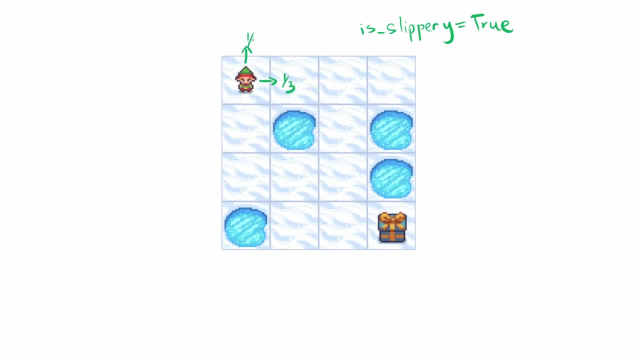 it will execute this action and there's a two-third chance of it going in an adjacent direction. Now, with Slippery turned on, pathfinding algorithm will not be able to solve this. In fact, I'm not even sure what it's going to do, So I'm going to use a pathfinding algorithm to solve this. 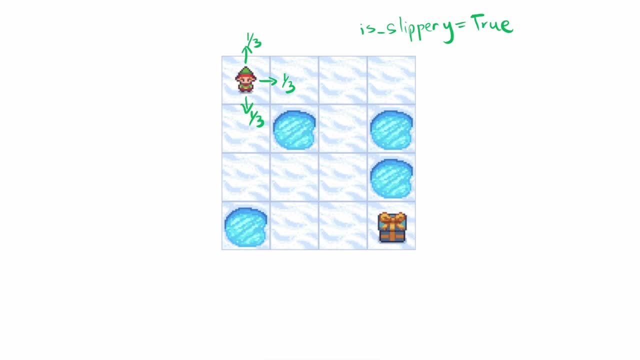 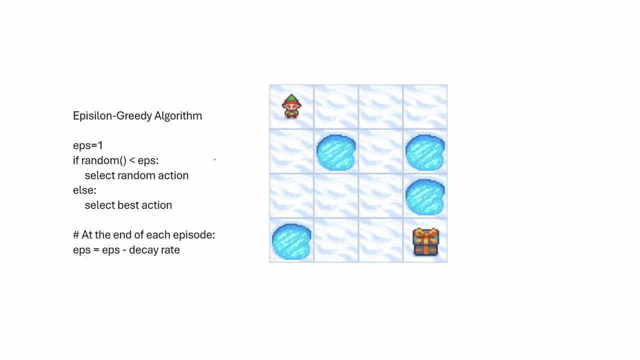 If I don't know how to solve this, I can just give the agent some incentive and let it figure out how to solve this. So that's where reinforcement learning shines, In terms of how the agent navigates the map- both deep Q-learning and Q-learning, uses the 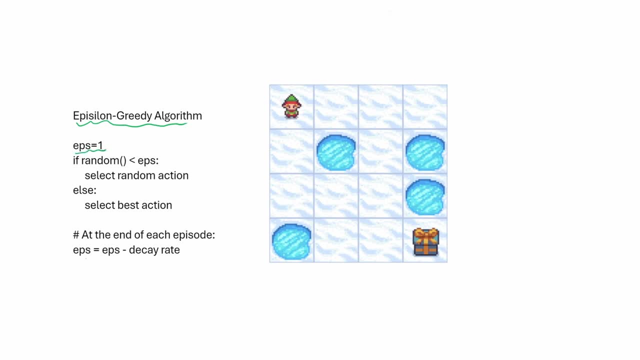 epsilon greedy algorithm. Basically, we start with a variable called epsilon equal and set it equal to one, And then we just give the agent some incentive and let it figure out how to solve this, And then we generate a random number If the random number is less than epsilon. 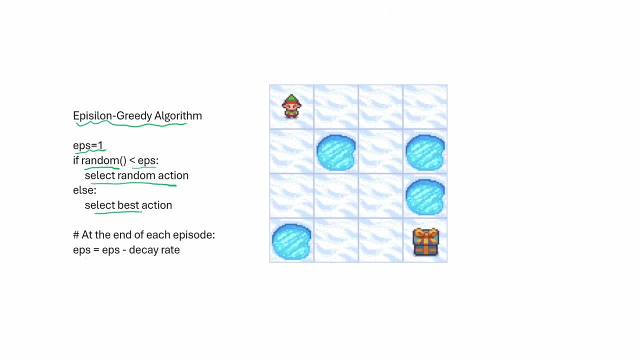 we pick a random action. Otherwise we pick the best action that we know of at the moment, And at the end of each episode we'll decrease epsilon by a little bit at a time. So essentially we start off with 100% random exploration and then eventually near the end of training. 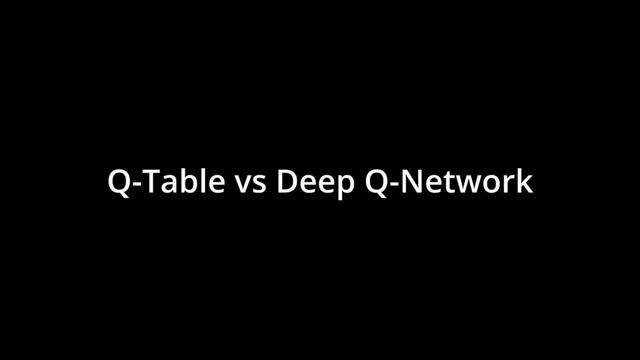 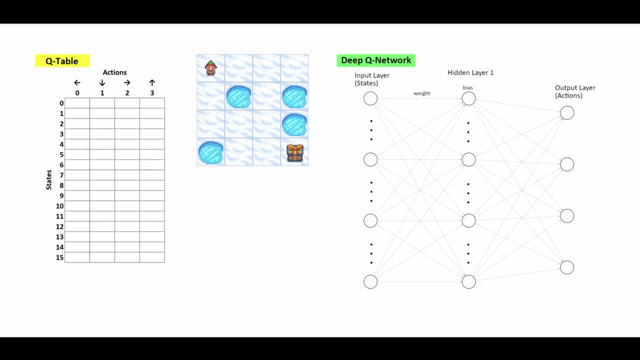 we're going to be always selecting the best action to take. Before we jump into the details of how the training works between Q-learning versus deep Q-learning, let's take a look at what the outcome looks like For Q-learning. the output of the 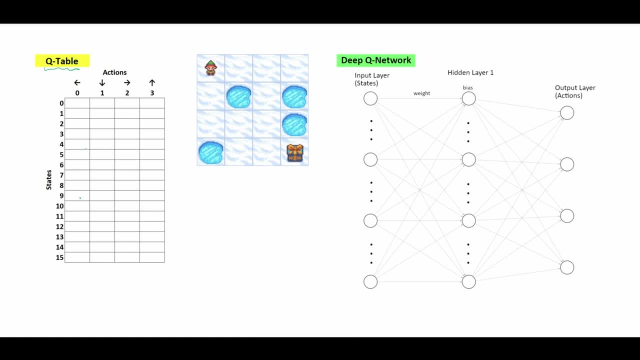 training is a Q-table, which is nothing more than a two-dimensional array consisting of 16 states by four actions. After training, the whole table is going to be filled with Q-values. For example, it might look something like this: So in this case, the agent is at state zero. We look at the table and see what the maximum value 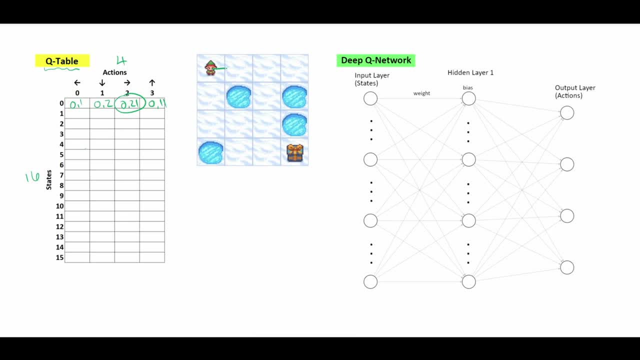 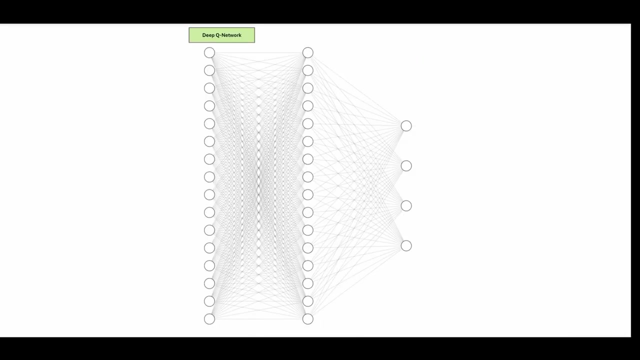 is. In this case, it's to-go-right. So this is the prescribed action over at deep Q-learning. The output is a deep Q network, which is actually nothing more than a regular feedforward neural network. This is actually what it looks like, but I think we should switch back to the simplified 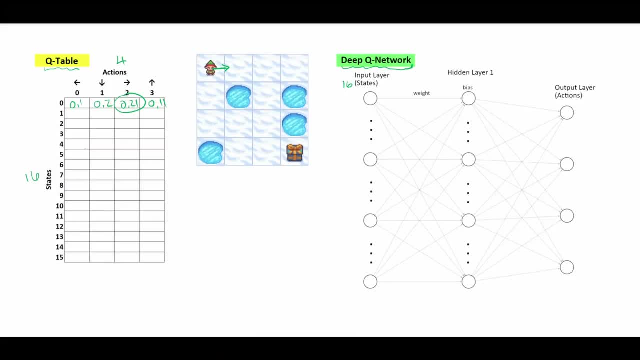 view. the input layer is going to have 16 nodes. the output layer is going to have four nodes. the way that we send an input into the input layer is like this: if the agent is at state 0, we're going to set the first node to 1 and everything else 0. if the agent is at state 1: 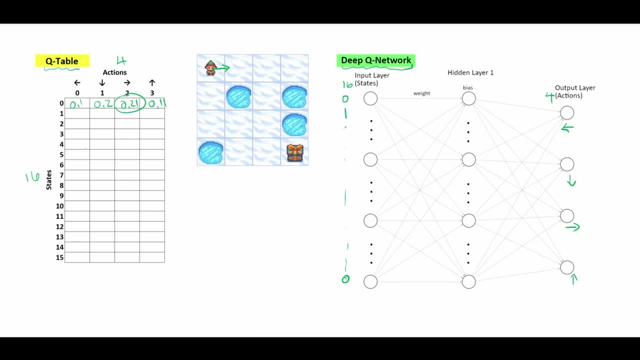 then the first node is 0 and the second node is 1 and everything else is 0. so this is called one hot encoding. just do one more, if it's at the last. if we want to put in state 15, then everything are zeros and state 15 is 1.. so that's how the input works. with the input, the output that gets. 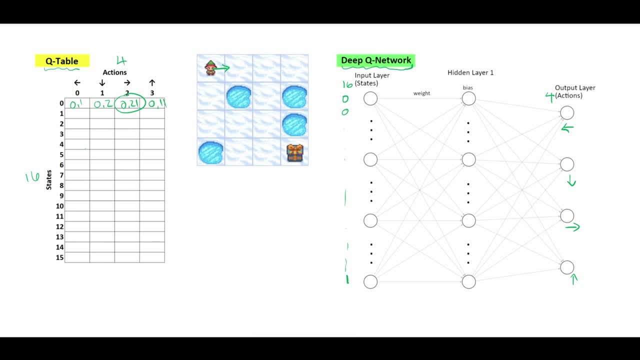 calculated are q values. now, the q values are not going to look like what's in the q table, but it might be something similar. let me throw some numbers in here, okay. so same thing for this particular input. the best action is the highest q value. when training a neural network, essentially we're trying to train the weights associated with each. 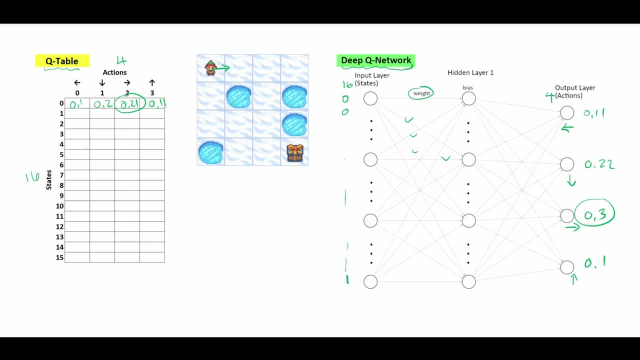 one of these lines in the neural network and the bias for all the hidden layers. now how do we know how many hidden layers we need? in this case, one layer was enough, but you can certainly add more if necessary- and how many nodes do we need in the hidden layer? i try 16 and it's able to solve the map. so 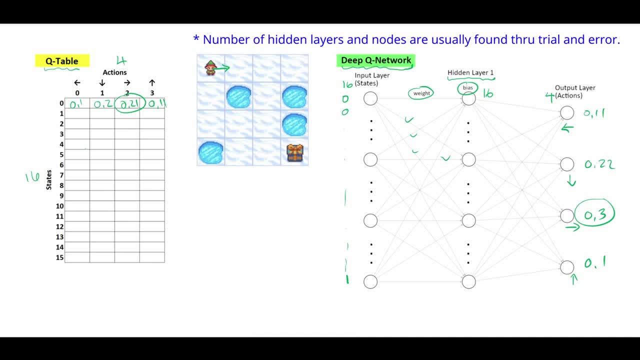 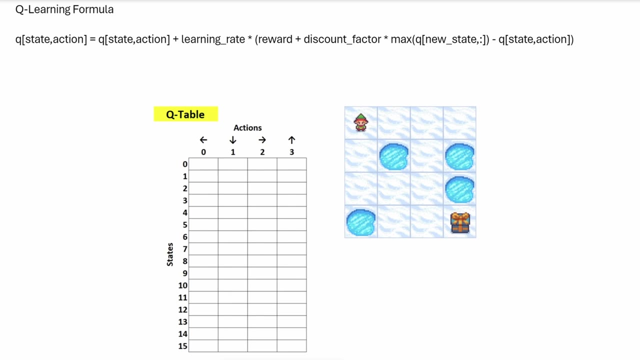 i'm sticking with that, but you can certainly increase or decrease this number to see what happens. okay, so that's the differences between the output of q learning versus deepq learning. as the agent navigates the map, it is using the q learning formula to calculate the q values and update the q table. now the 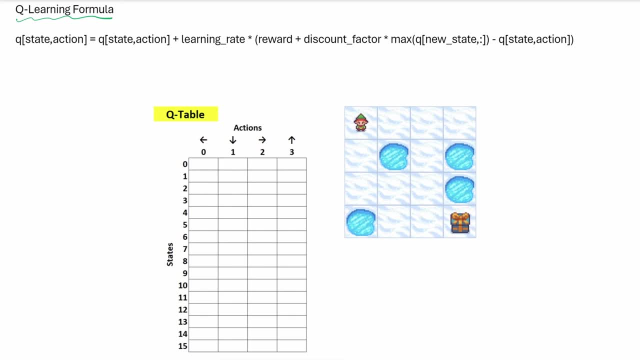 formula might look a little bit scary, but it's actually not that bad. let's work through some examples. let's say our agent is in state 14 and it's going right to get to state 15.. we're calculating q of state 14, action 2, which is this cell. 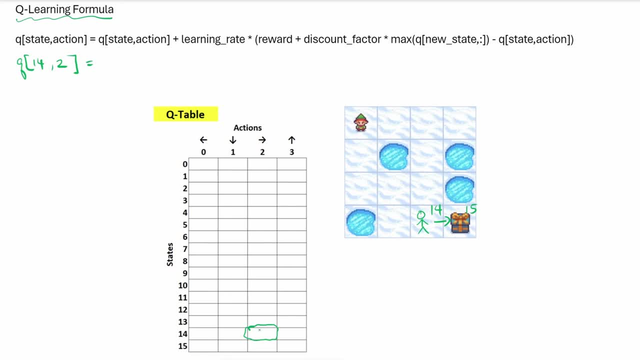 the current value of that cell is 0 because we initialized the whole Q table to 0 at the beginning, plus the learning rate. the learning rate is a hyper parameter that we can set. as an example, I'll just put in 0.01 times the reward. 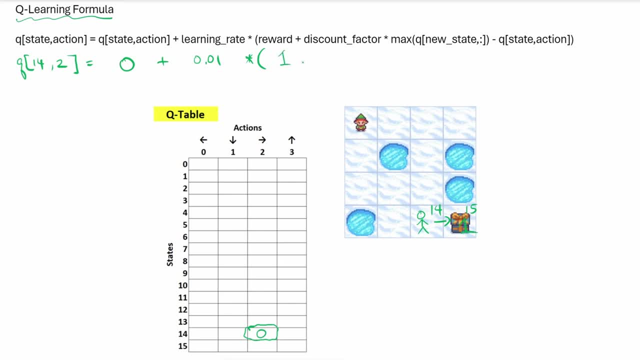 we get a reward of 1 because we reached the goal, plus the discount factor, another parameter that we set. I'll just use 0.9 times the max Q value of the new state, so the max Q value of state 15, since state 15 is a terminal state, it. 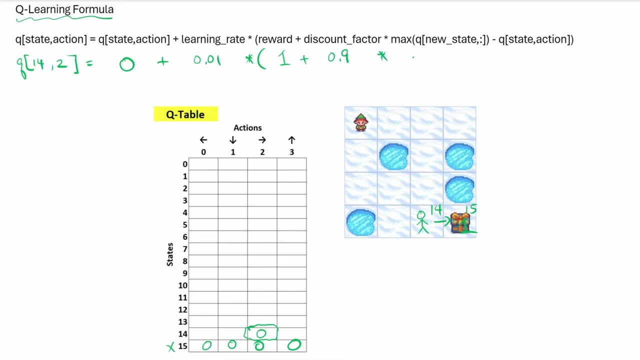 will never get anything other than zeros in this table. max is 0. essentially, these two are gone subtracted by the same thing that we had here. okay, so walk through the math: this is just 0.01. so we get 0.01 here. now let's do another one really quickly. agent is here. take a right Q of 13 going. 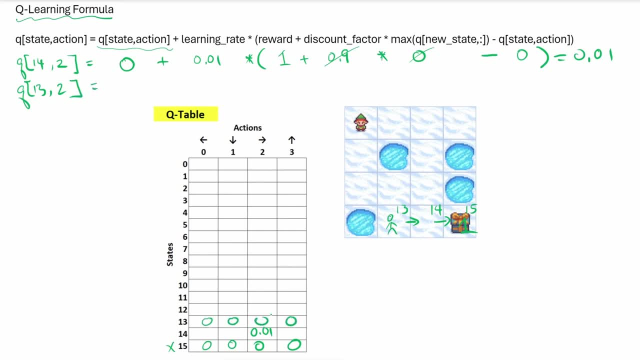 to the right. 13 is also all zeros. this is the one we're updating here is 0 plus the learning rate rate times a reward: there is no reward plus the discount factor times max of the new state. max of state 14. max of state 14 is 0.01. subtracted by again, it's zero. this is equal to 0.009. okay, it's. 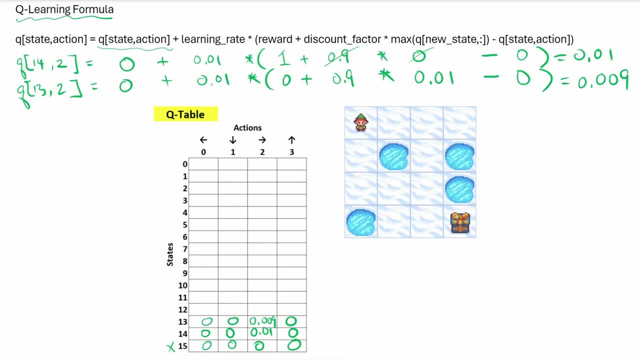 actually pretty straightforward. now how the heck does this formula help find a path? so if we train enough, the theory is that this number is going to be really close to one, and then the states next to it- it's gonna be 0.9 something. and then the states adjacent to that: it's probably going to be 0.8. 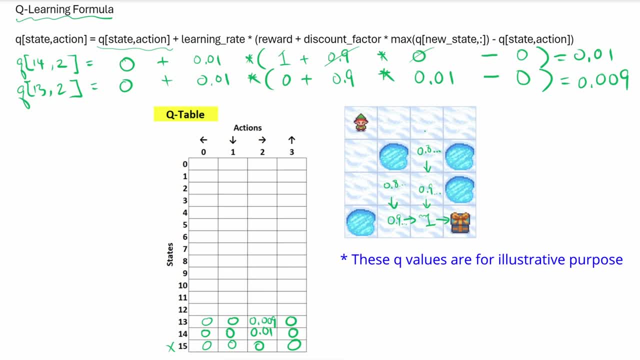 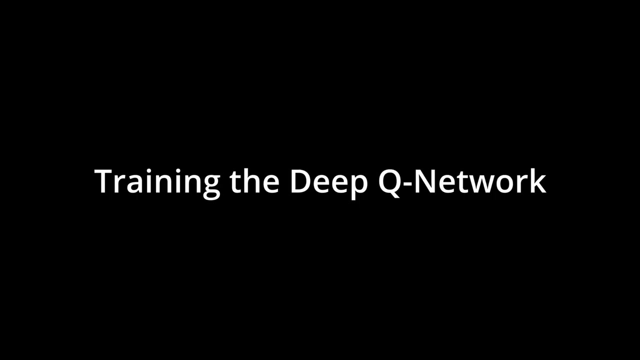 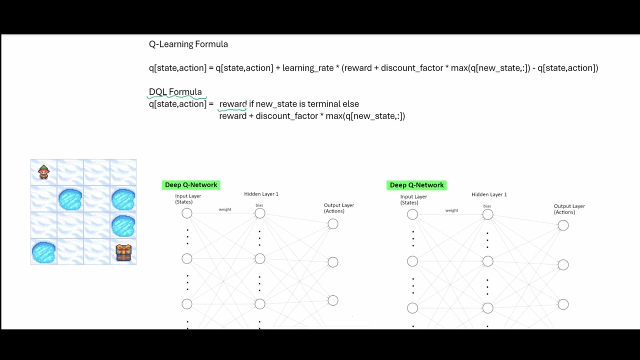 something, and if we keep going, we can see that a path is actually two paths are possible. so mathematically, this is how the path is found. over at deepq learning, the formula is going to look like this: we are going to create a path with the key of q equal to the reward. 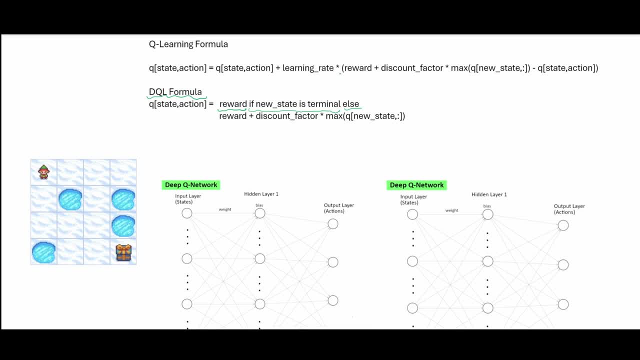 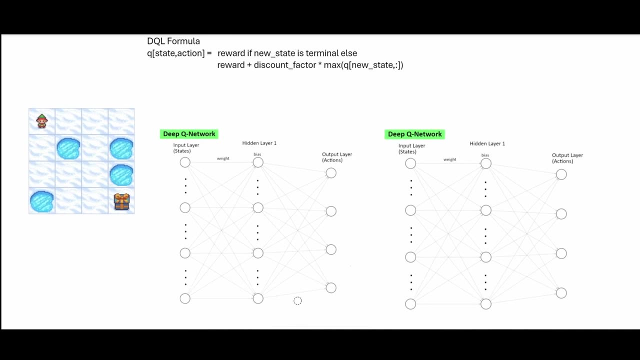 if the new state is a terminal state. otherwise we set it to this part of the q-learning formula. let's see how the formula is going to be used in training for deepq learning. we actually need two neural networks. let me walk through the steps. the network on the left: 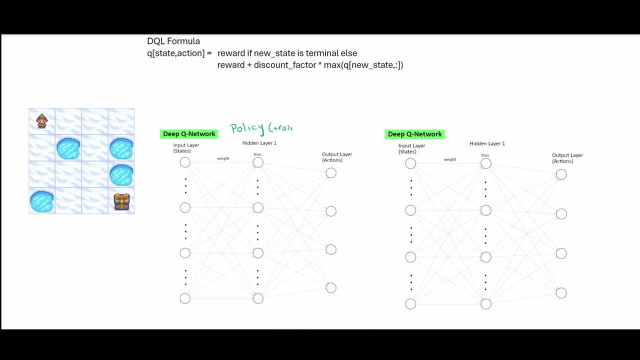 policy network. This is the network that we're going to do the training on. The one on the right is called the target network. The target network is the one that makes use of the DQ learning formula. Now let's walk through the steps of training. Step one is going to be creation of 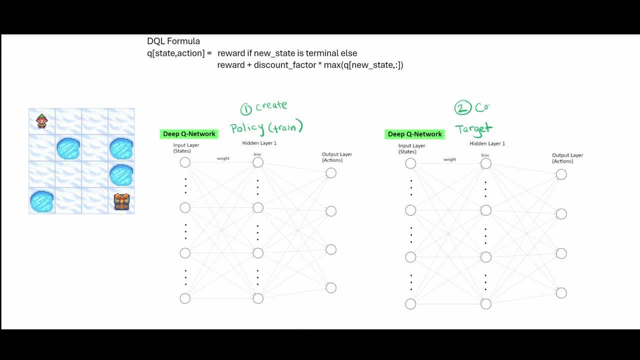 this policy network. Step two: we make a copy of the policy network into the target network. So basically we're copying the weights and the bias over here, So both networks are identical. Step number three: the agent navigates the map as usual. Let's say the agent is here in state 14. 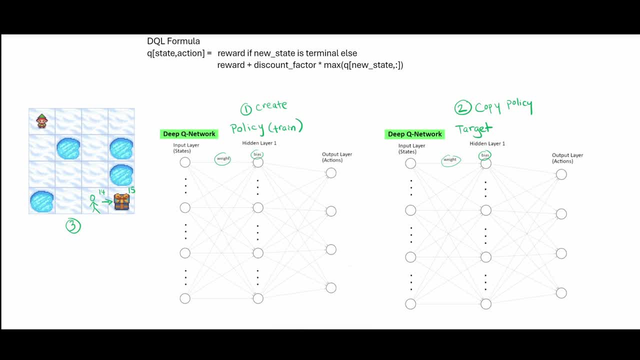 and it's going into state 15.. Step three is just navigation. Now step four: we input state 14.. Remember how we have to encode the input. It's going to look like this: Zero One, two, three, Twelve thirteen. 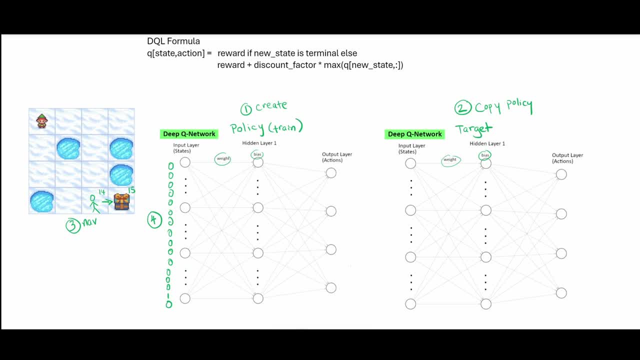 State 14.. Fifteen, The input is going to look like this. As you know, neural networks, when it's created it comes with a random set of weights and bias. So with this input we're actually going to get an output, even though these values are pretty much meaningless. So we might get some stuff that 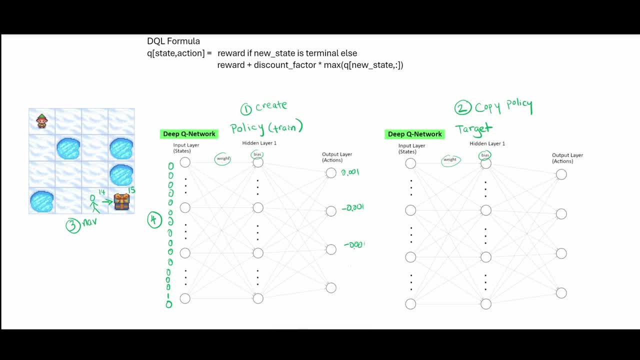 looks like I'm just putting in some random numbers. Okay, So these Q values are meaningless. And as a reminder, this is the left action, down, right and up. Okay, Step five. we do the same thing, We take. 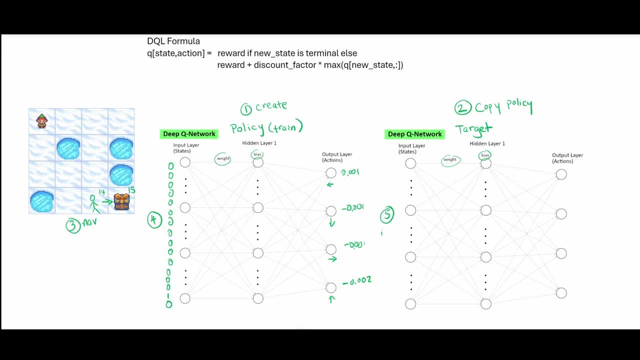 the exact same input- state 14, and send it into the target network, which will also calculate the exact same numbers, because the target network is the same as the policy network currently. Step six: This is where we calculate the Q value for state 14.. We're taking the action of two is 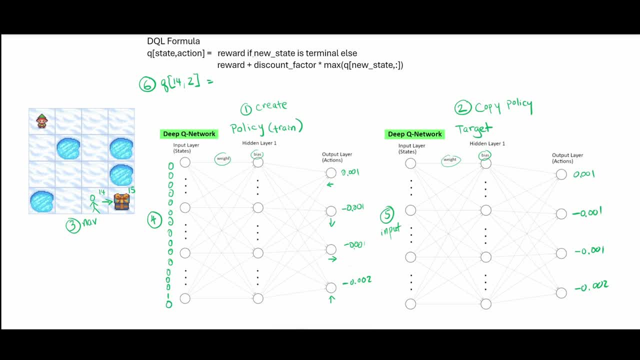 equal to, since we're going into state 15.. It is a terminal state. We set it equal to one step. seven, All right. So that's the first step. The last is to get the biased the best value to the target. 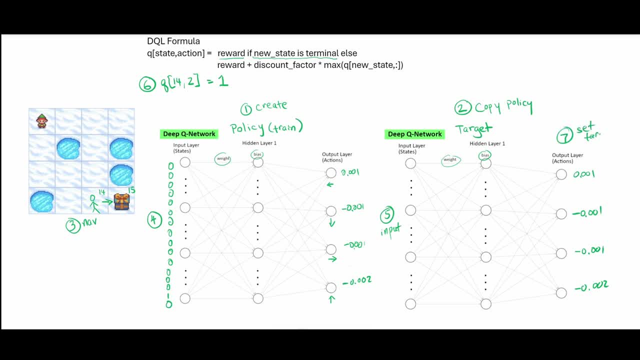 Step 7 is to set the target Input. state 14, output. action 2 is this node. We take the value that we calculated up on step 6 and we replace the Q value in the output. Step number 8, we take the target Q values. we'll use it to train the policy network. 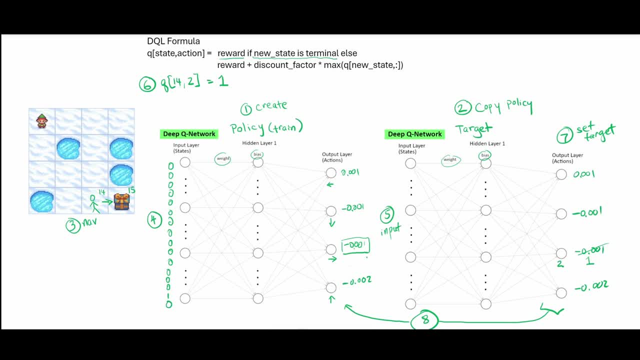 So this value is the one that's really going to change. As you know, with neural networks it doesn't go straight to 1, it's going to go toward that direction. So maybe, maybe it'll go to 0.01.. 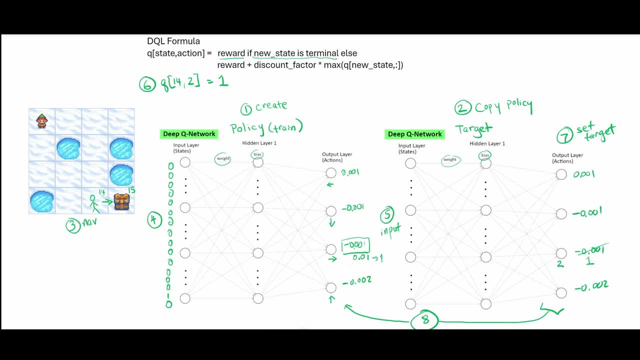 But if you repeat the training many, many times, it will approach 1.. Step 9 is to repeat the whole thing again. Of course we're not going to create the policy network, we're not going to make a copy of it. 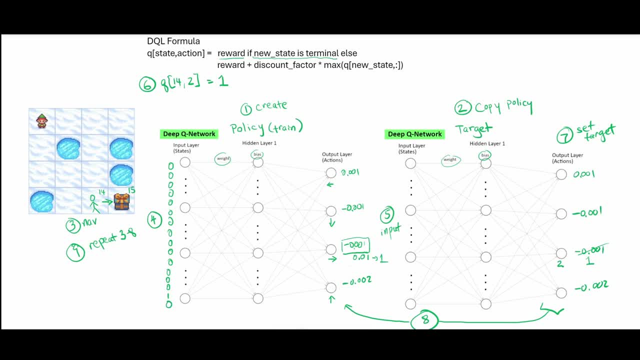 So what we're repeating Is steps 3 through 8.. Step 10,, after a certain number of steps or episodes, we're going to sync the policy network with the target network, which means we're going to make them identical by copying the. 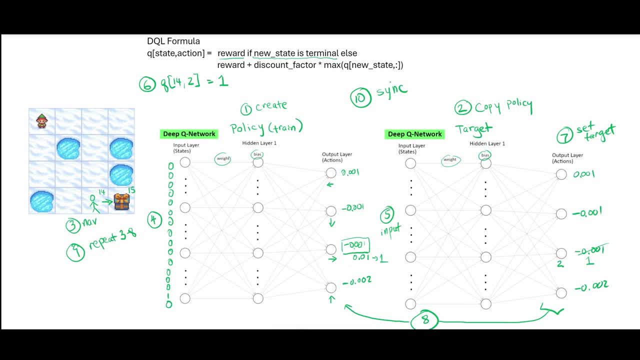 weight and biases from the policy over to the target network. After syncing the networks, we're going to repeat 9 again and then repeat 10 until training is done. Okay, So that's generally how DeepQ looks. So let's see how DeepQ learning works. 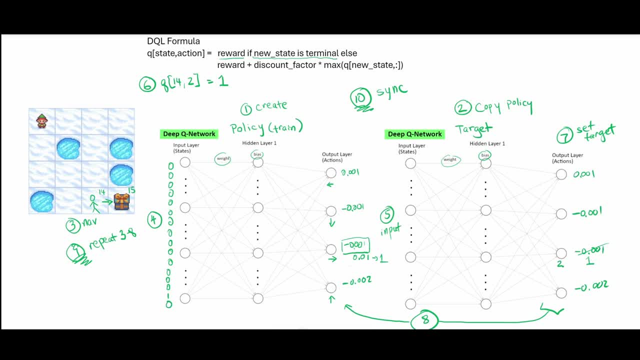 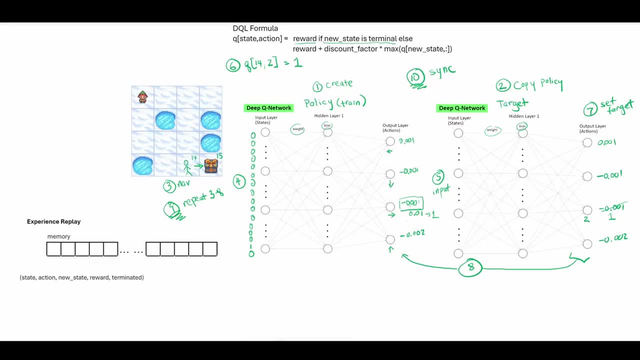 That might have been a little bit complicated, So maybe rewind the video, watch it again and make sure you understand what's happening. To effectively train a neural network, we need to randomize the training data that we send into the neural network. However, if you remember from steps 3 and 4, the agent takes an action and then we're. 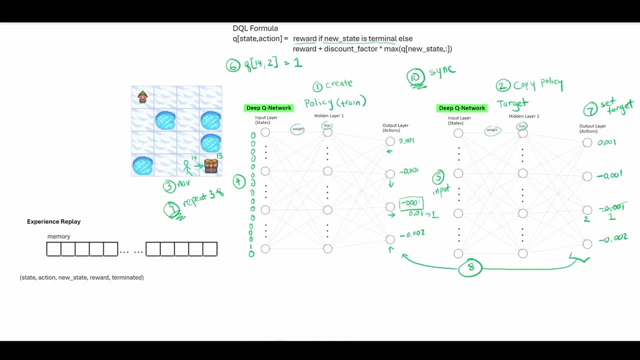 sending that training data into the neural network. So the question is: how do we? How do we? What is the order of a single sample? Well, that's where experience replay comes in. We need a step 3a where we memorize the agent's experience. 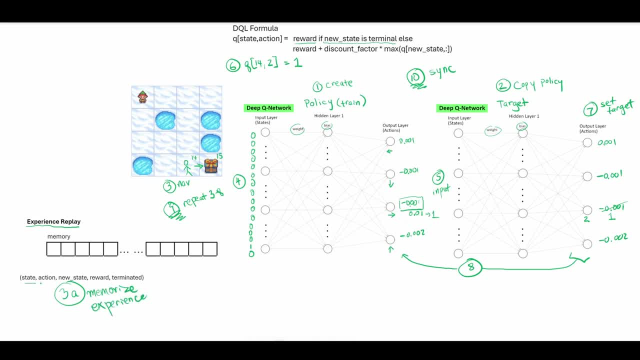 As the agent navigates the map, we're storing the state that it was, in what action it took, the new state that it reached, if there was a reward or not, and if the new state is a terminal state or not. We take that and insert it into the memory, and the memory is nothing more than a Python. 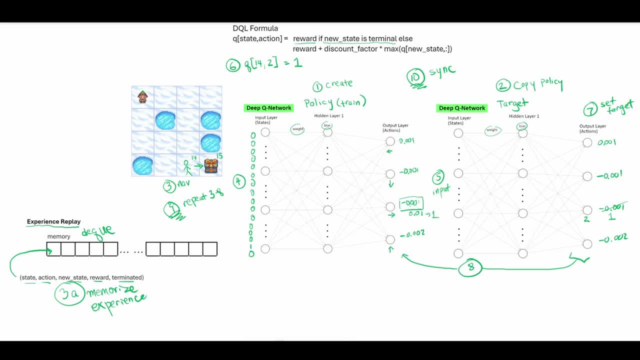 deck. How a deck works is that as the deck gets full, whatever at the end gets purged. We need a step 3b. This is the replay step. This is where we take, say, 30 random samples from the deck and then pass it on to step 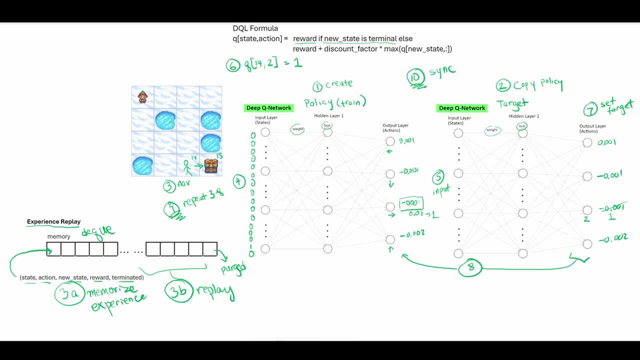 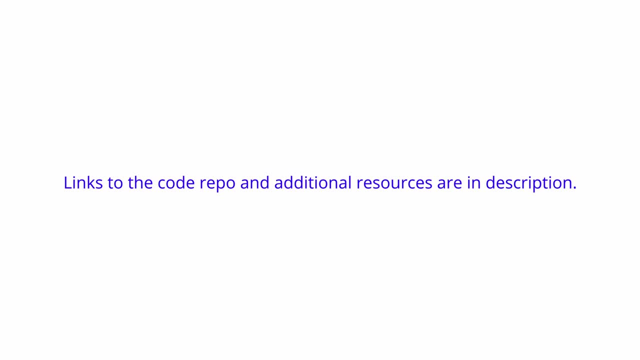 4 for training. So that's what experience replay is Before we jump into the code. if you have problems installing Genasium, explore the code. If you have problems installing Genasium, explore the code. If you have problems installing Genasium, explore the code. 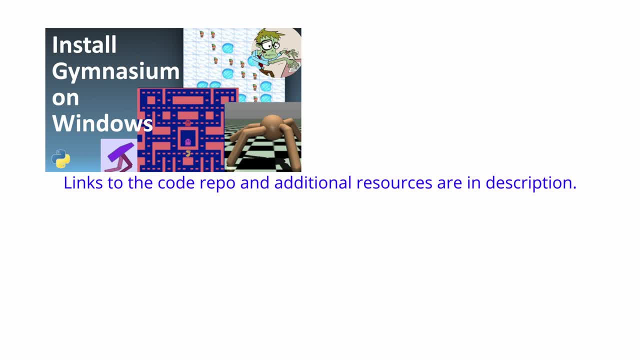 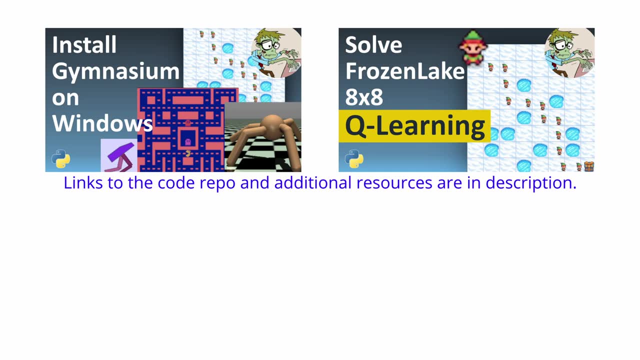 I'm not going to walk through the Q-learning code, but if you are interested in that, jump to my Q-learning code walkthrough video after watching this one. Also, if you have zero experience with neural networks, you can check out this basic tutorial. 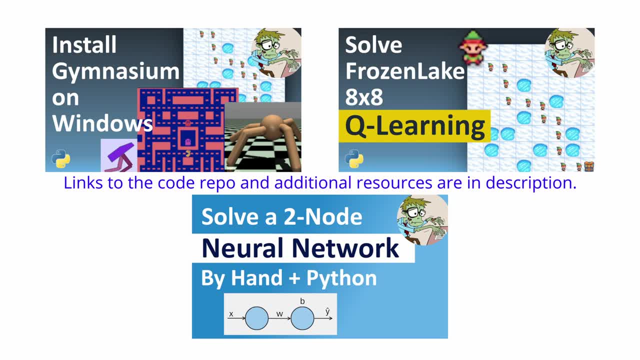 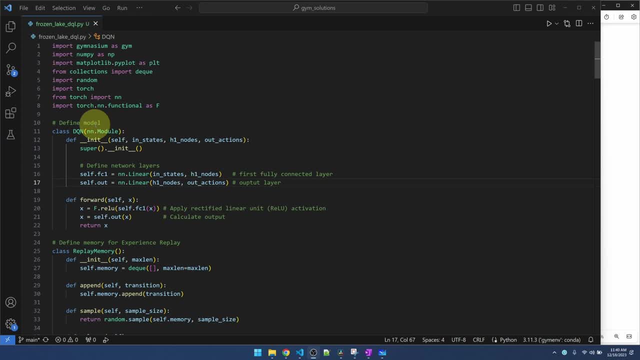 on neural networks. You also need PyTorch, so head over to pytorchorg and get that installed. The first thing that we do is create a class to represent our DeepQL network. I'm calling it DeepQLNetwork. I'm calling it DQN. 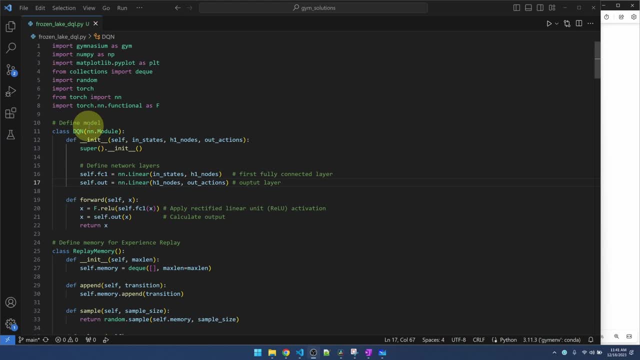 As mentioned before, a DeepQ network is nothing more than a feedforward neural network, So there's really nothing special about it. Here I'm using a pretty standard way of creating a neural network using PyTorch. If you look up any PyTorch tutorial, you'll probably see something just like this. 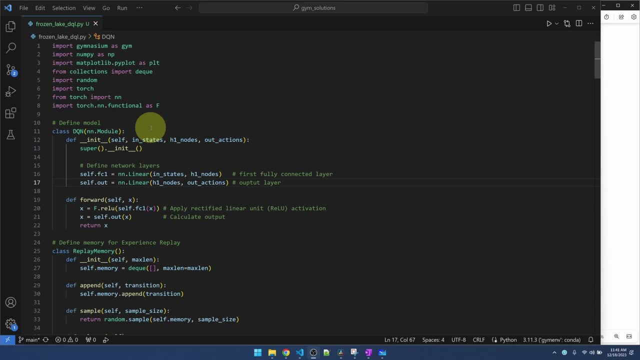 So, since this is not a PyTorch tutorial, I'm not going to spend too much time explaining how PyTorch works. For this class, we have to inherit the neural network module, which requires us to implement two functions: the init function and the forward function. 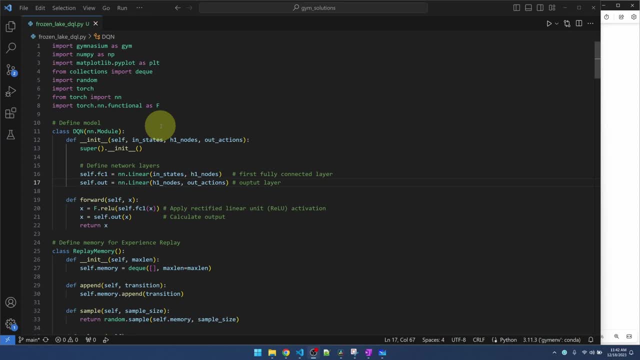 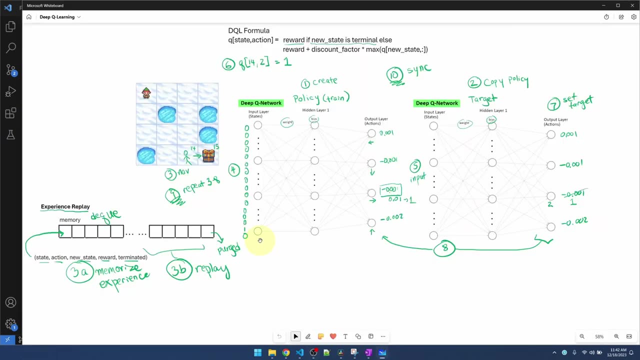 In the init function I'm passing in the number of nodes in my input state, hidden layer and output state. Back at our diagram. we're going to have 16 input states, As mentioned before. I'm using 16 in the hidden layer. 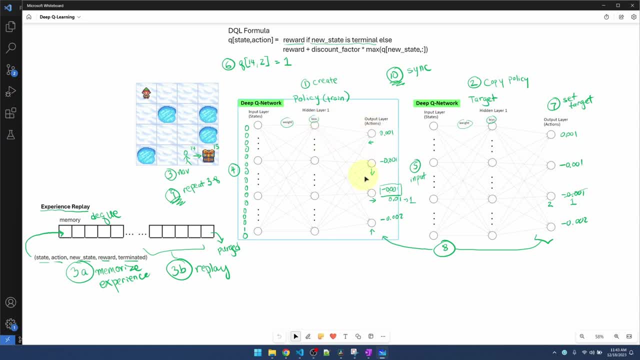 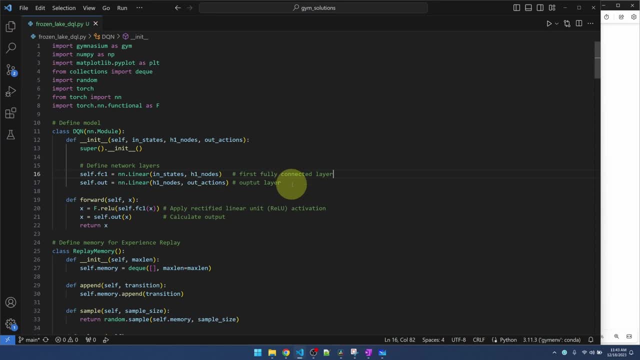 That's something that you can adjust yourself, And in the output layer we're going to declare four nodes. We declare the hidden layer, which has 16 going into 16, and then the output layer, 16 going into 4.. 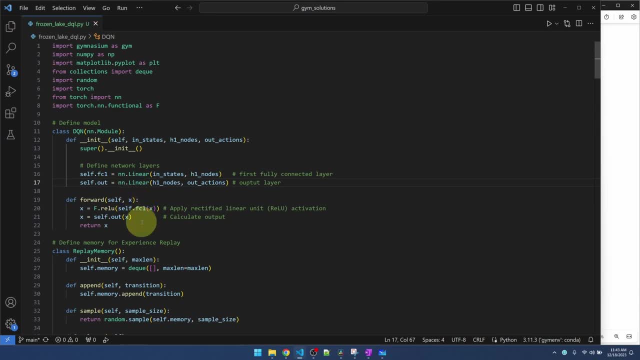 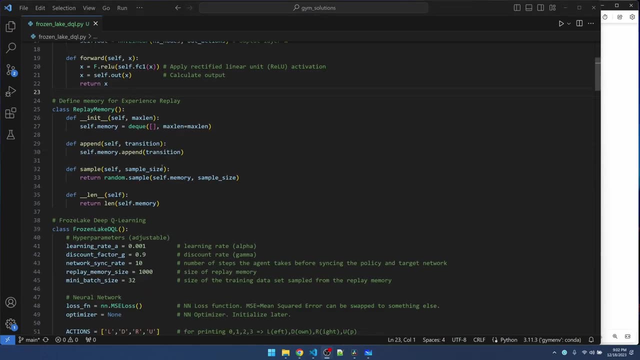 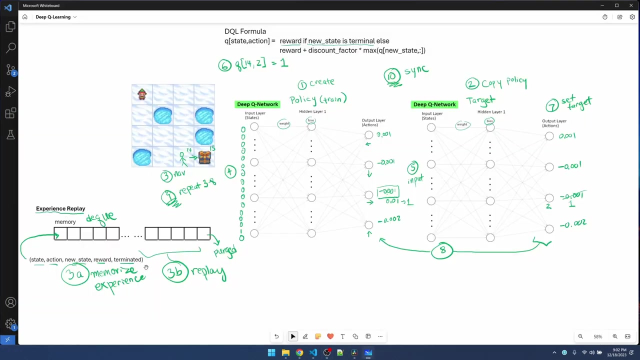 And then the forward function. x is the training data set, and we're sending the training data through the neural network. Again, this is pretty common PyTorch code. Next, we need a class to represent the replay memory. So it's this portion that we're implementing. 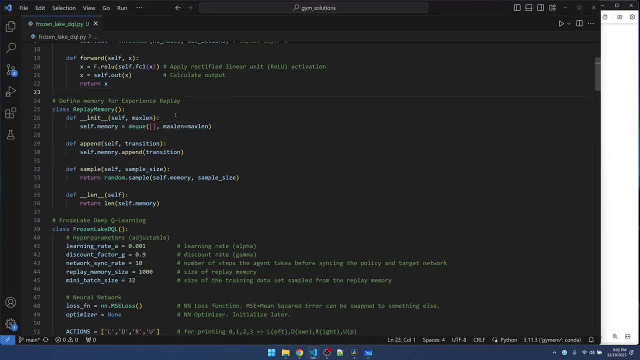 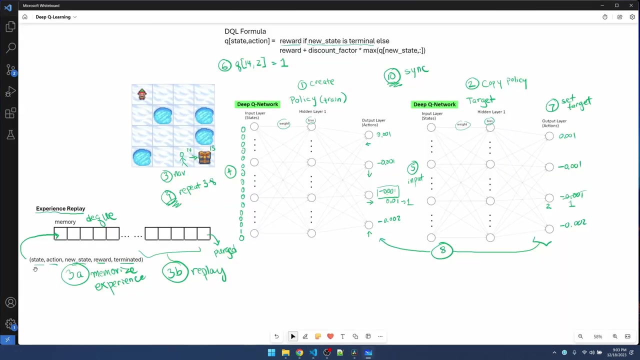 Right now in the init function we'll pass in a max length and then create the Python deck. In the append function we're going to append the transition. The transition is this tuple here: state, action, new state, reward and terminated. 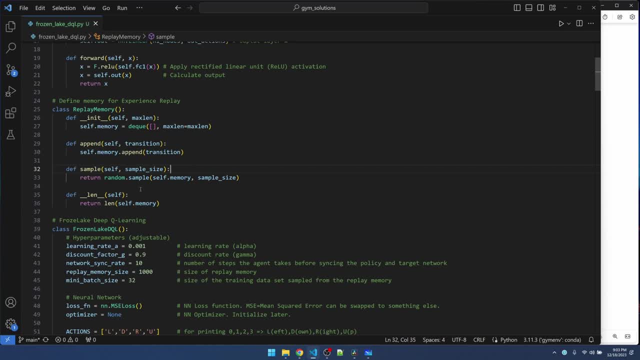 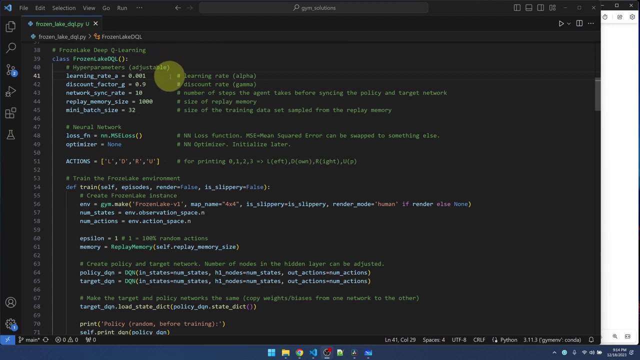 The sample function will return a random sample of whatever size we want from the memory, And then the link function simply returns the length of the memory. The Frozen Lake DQL class is where we're going to do our training. We set the learning rate and the discount factor. 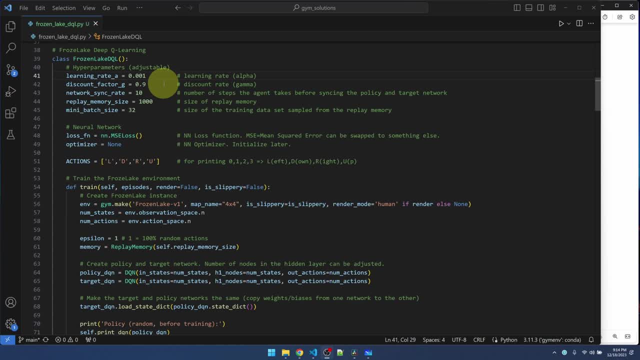 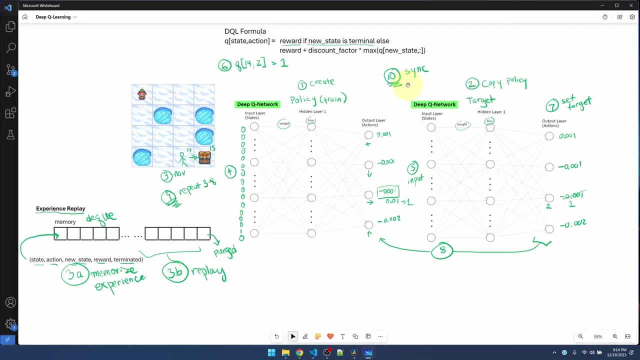 Those are part of the Q-learning formula And these are values that you can adjust and play around with The network sync rate, It's the number of steps the agent takes before syncing the policy and target network. That's the setting for step 10,. 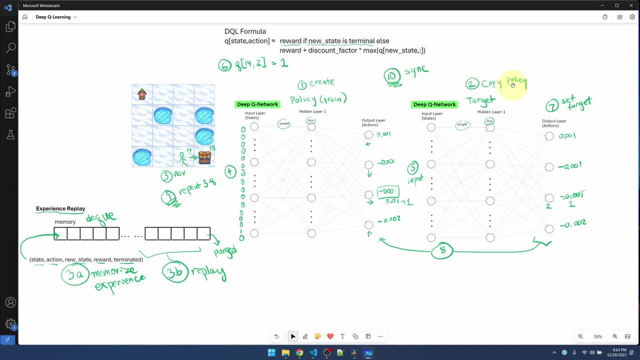 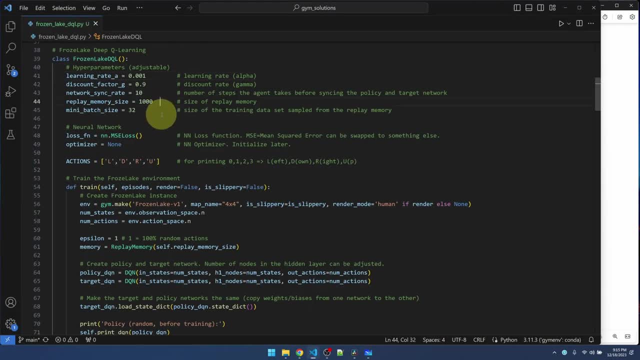 where we sync the policy and the target network. We set the replay memory size to 1000 and the replay memory sample size to 32.. These are also numbers that you can play around with. Next is the loss function and the optimizer. These two are PyTorch variables. 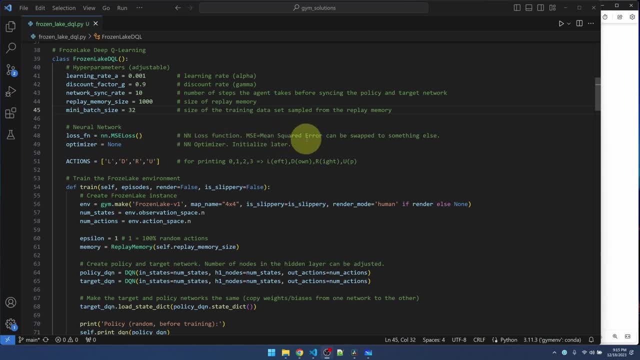 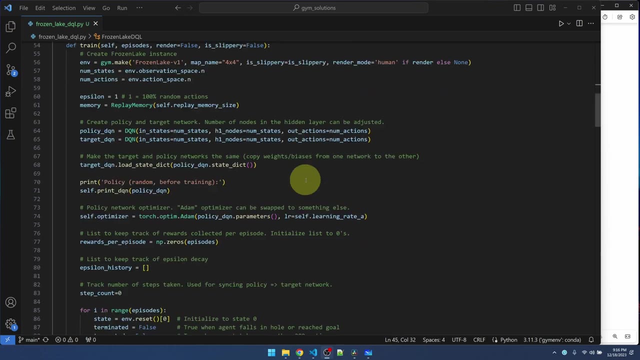 For the loss function, I'm simply using the mean square error function For the optimizer. we'll initialize that at a later time. This actions list is to simply map the action numbers into letters for printing. In the train function we can specify how many episodes we want to train the agent. 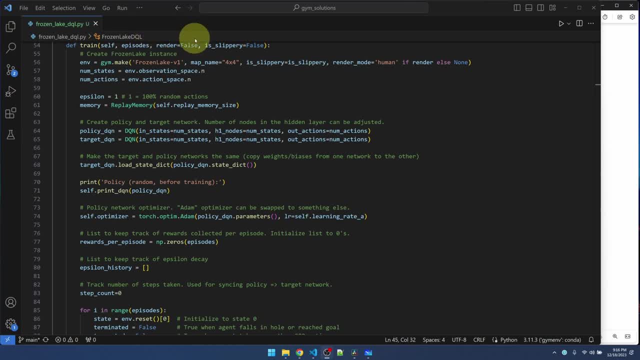 whether we want to render the map on screen and whether we want to turn on the slippery flag. We'll instantiate the frozen lake environment and then create a variable to store the number of states- This is going to be 16. And store the number of actions. 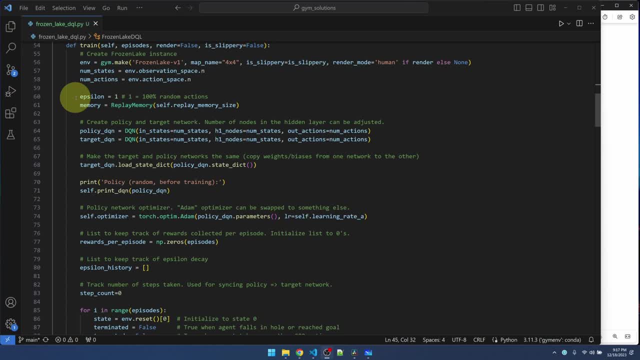 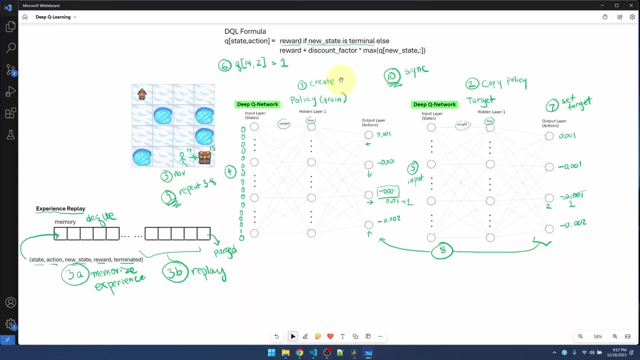 This is going to be 4.. Here we initialize epsilon to 1 and we instantiate the replay memory. This is going to be size of 1000.. Now we create the policy DQ network. This is step one. create the policy network. 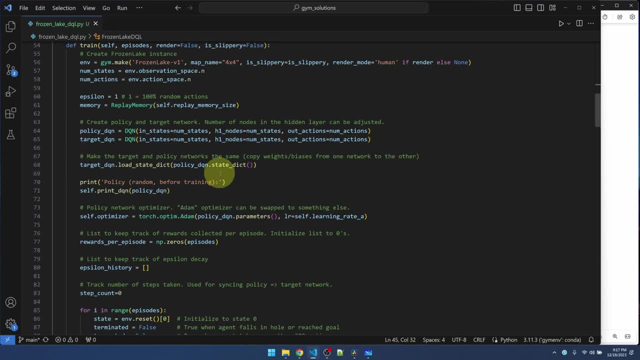 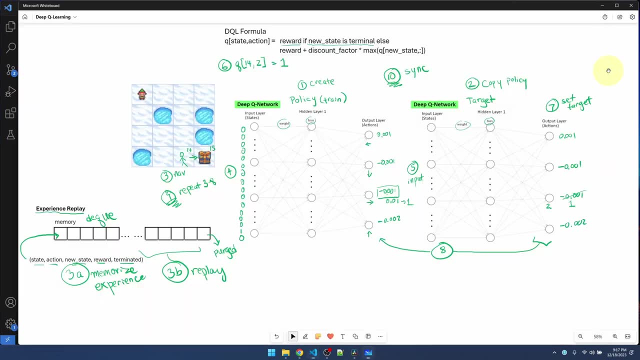 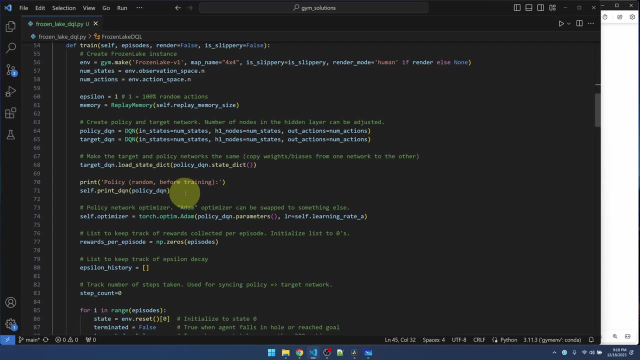 We also create a target network and copy the weights and bias from the policy network into the target network. So that is step number two, making the target and policy network identical. Before training we'll do a printout of the policy network just so we can compare it to the end result. 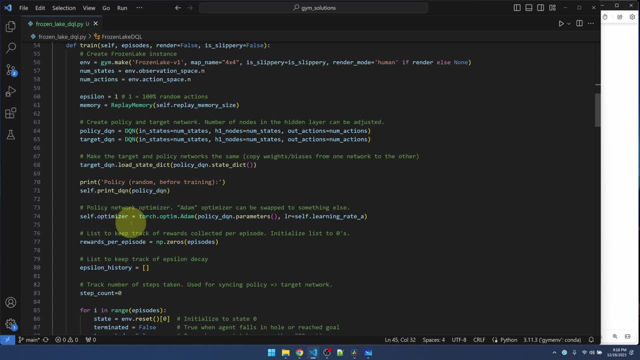 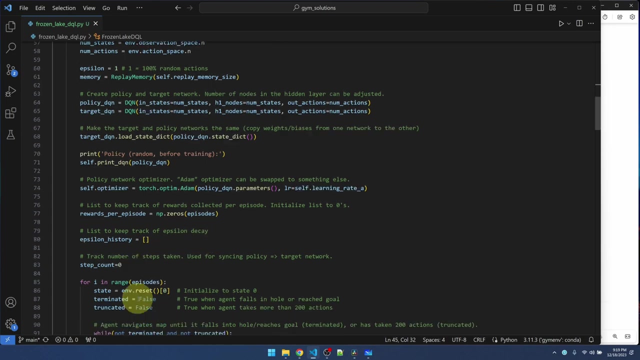 Next, we initialize the optimizer that we declared earlier And we're simply using the atom optimizer passing in the learning rate. We'll use this rewards per episode list to keep track of the rewards collected per episode. We'll also use this epsilon history list to keep track of epsilon decaying over time. 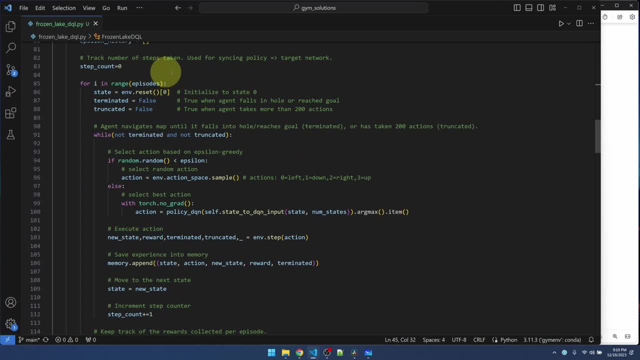 We'll use step count to keep track of the number of steps taken. This is used to determine when to sync the policy and target network again. So that is for step 10, the syncing. Next we'll loop through the number of episodes that were specified when calling the train function. 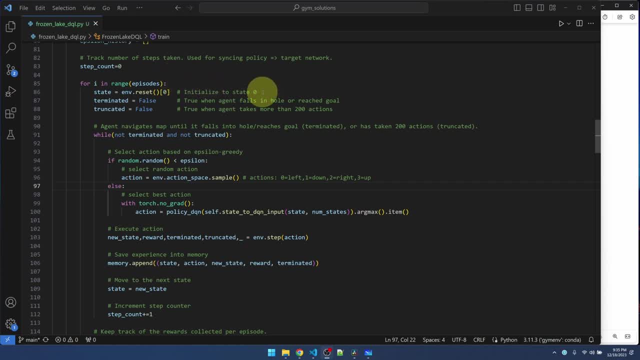 We'll initialize the map, So the agent starts at state zero. We'll initialize the terminated and truncated flag. Terminated is when the agent falls into the hole or reaches the goal. Truncated is when the agent takes more than 200 actions. 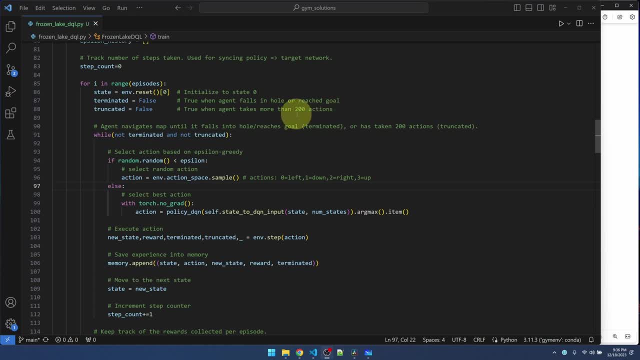 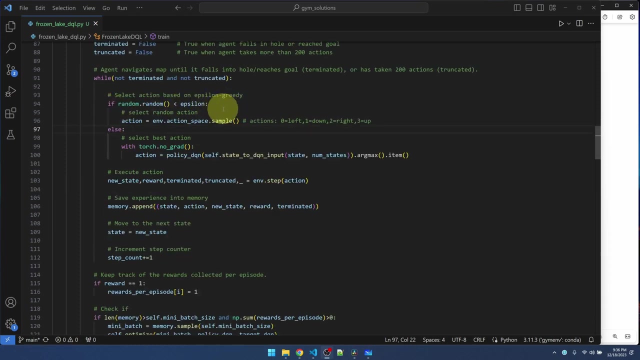 On such a small map- 4x4,. this is probably never going to occur, but we'll keep this anyway. Now we have a while loop checking for the terminated and truncated flag. Keep looping until these conditions are met. This part is basically the epsilon greedy algorithm. 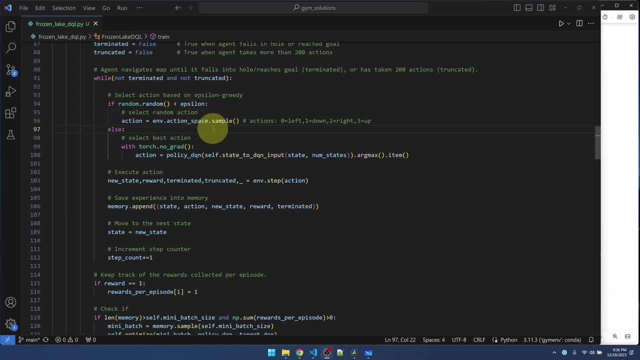 If a random number is less than epsilon, we'll just pick a random action. Otherwise, we'll use the policy network to calculate the set of Q values. take the maximum of that, extract that item and that's going to be the best action. 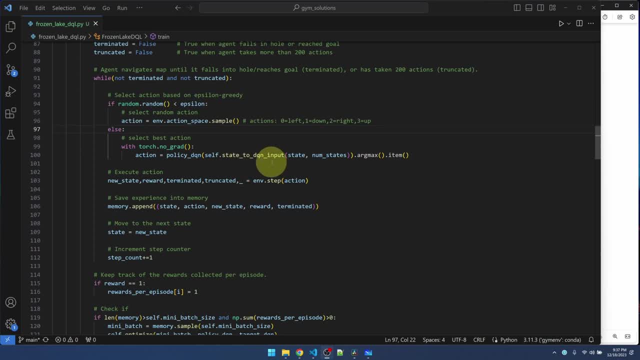 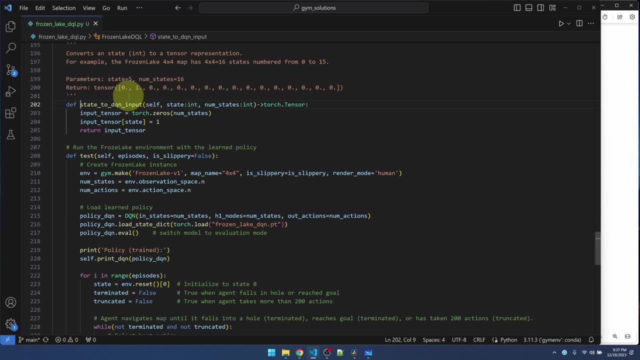 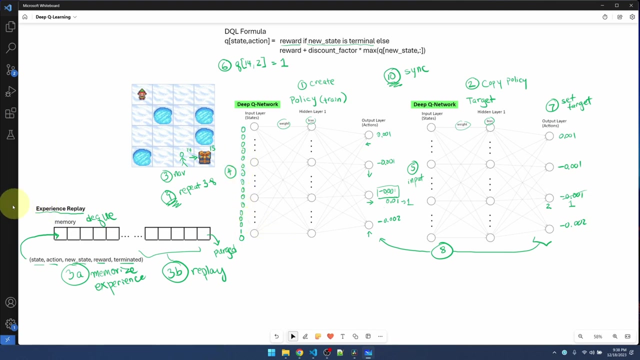 So we have a function here called state to DQN input. Let's jump down there. Remember that we have to take the state and encode it. That's what this function does, This type of encoding here. Okay, let's go back. 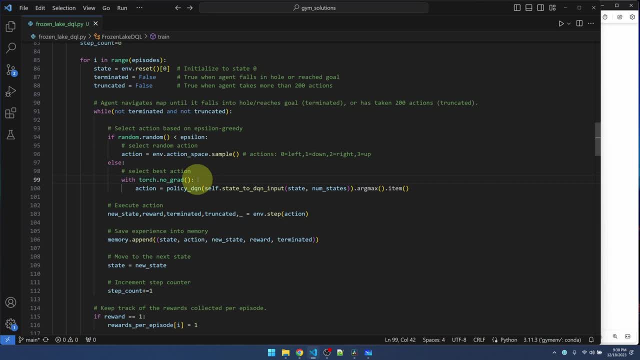 With PyTorch, we're going to perform a prediction. We should call this torchnoGrad so that it doesn't calculate the stuff needed for training. After selecting either a random action or the best action, we'll call the step function to execute the action. 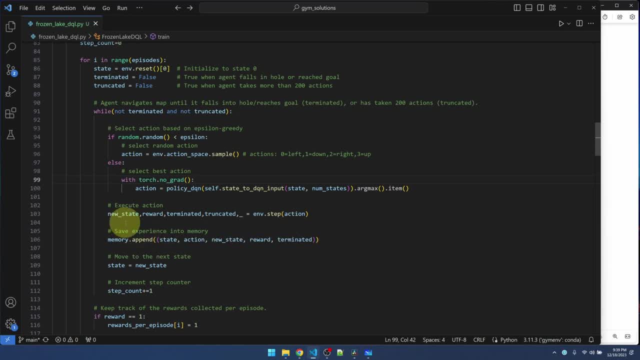 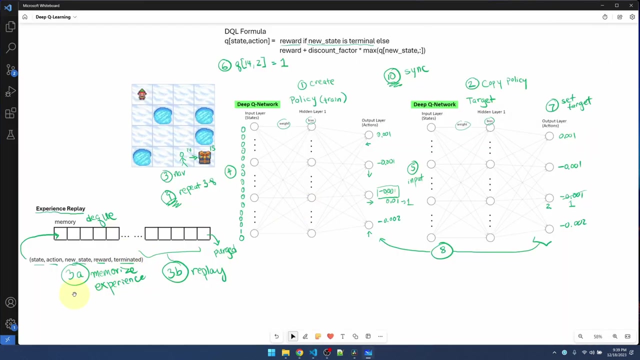 When we take that action, it's going to return the new state, whether there is a reward or not, whether it's a terminal state or we got truncated. We take all that information and put it into our memory. So that is step 3a. 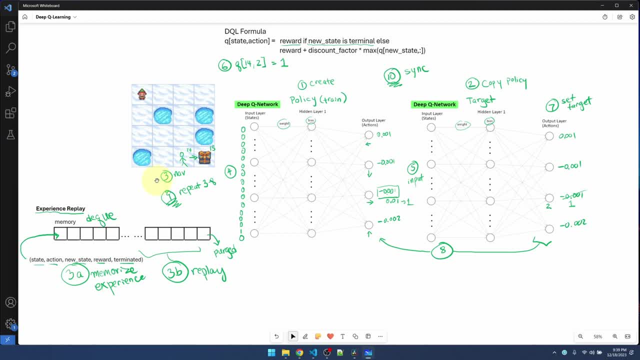 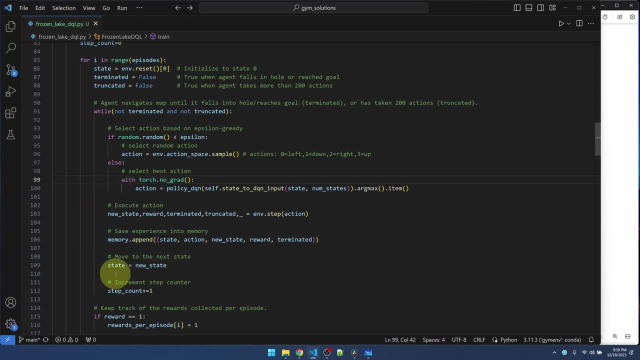 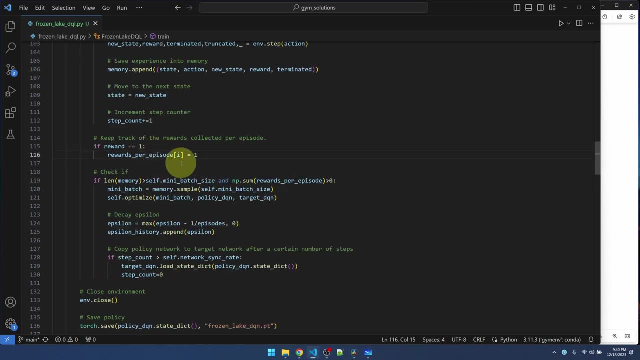 When we did the epsilon greedy, that was the step 3.. After executing the action, we're resetting the state equal to the new state. We increment our step counter. If we received an award, put it on our list Now. we'll check the memory. 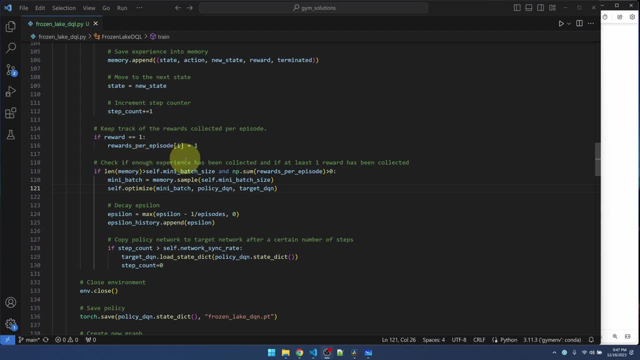 to see if we have enough training data to do optimization on. Also, we want to check if we have collected at least one reward. If we haven't collected any rewards, there's really no point in optimizing the network If those conditions are met. 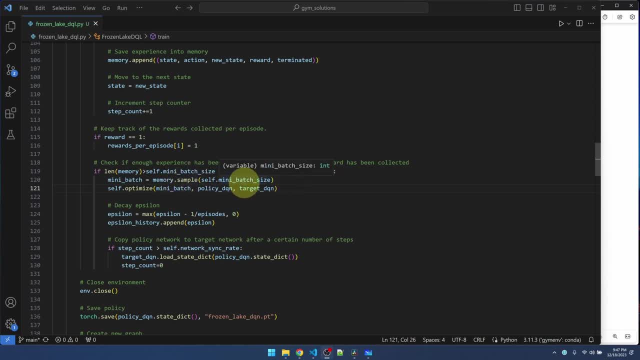 we use memorysample and we pass in the batch size, which was 32, and we get a batch of training data out of the memory. We'll pass that training data into the optimize function along with the policy network and the target network. Let's jump over to the optimize function. 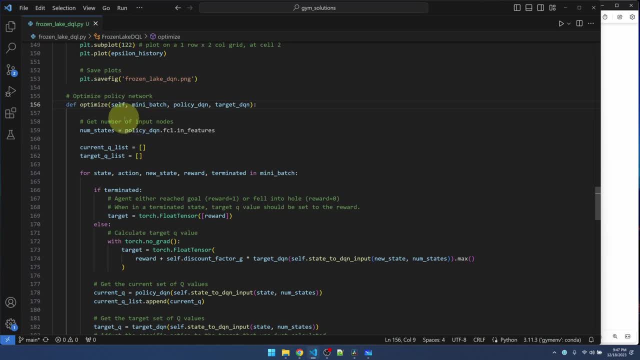 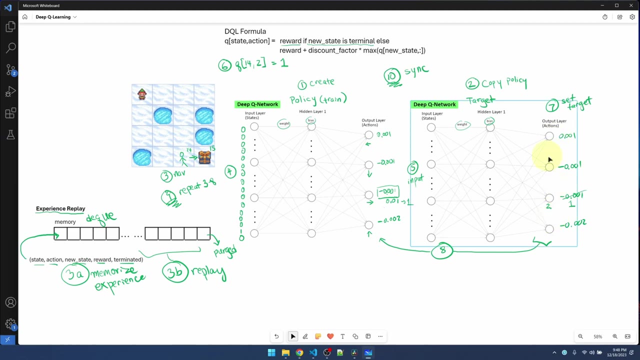 This first line is just looking at the policy network and getting the number of input nodes. We expect this to be 16.. The current queue list and target queue list. So this is the current queue list. This is the target queue list, What I'm about to describe now. 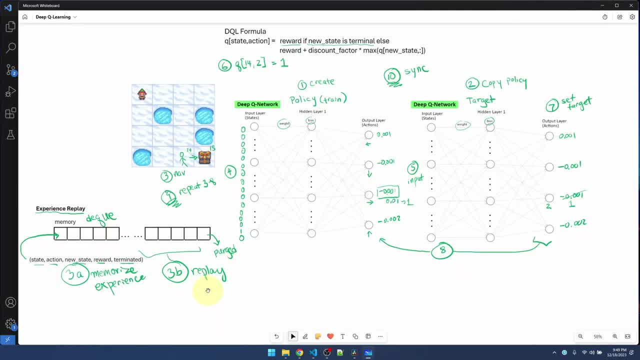 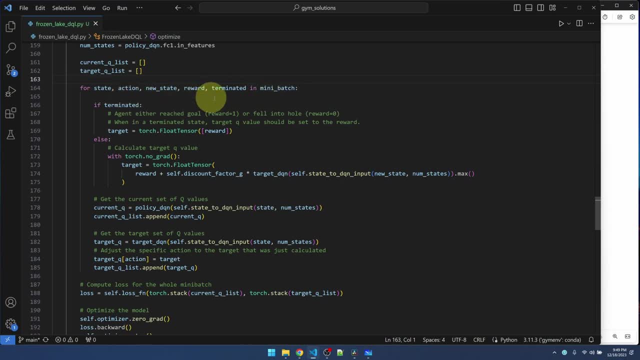 is step 3b: replaying the experience. So, to replay the experience, we're looping through the training data inside the mini-batch. Let's jump down here for a moment. So this is step number 4.. We're taking the states. 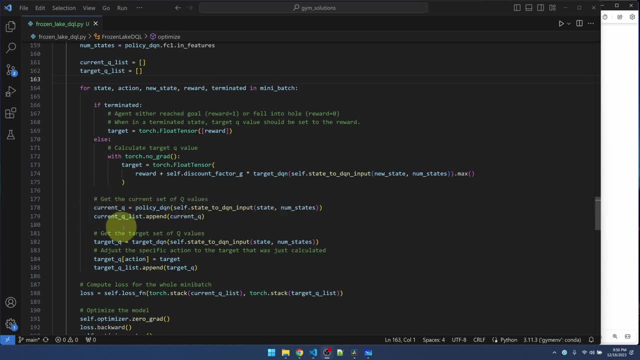 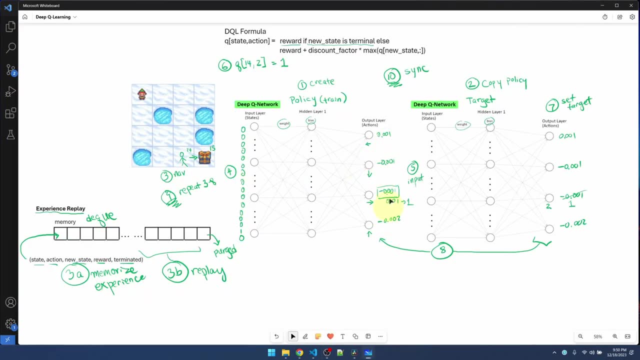 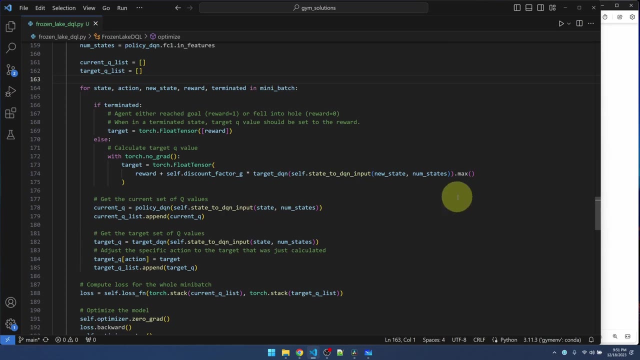 and passing it into the policy network to calculate the current list of queue values, Step number 4.. The output is the list of queue values, Step number 5.. We pass in the same thing to the target network, Step 5. We get the queue values out here. 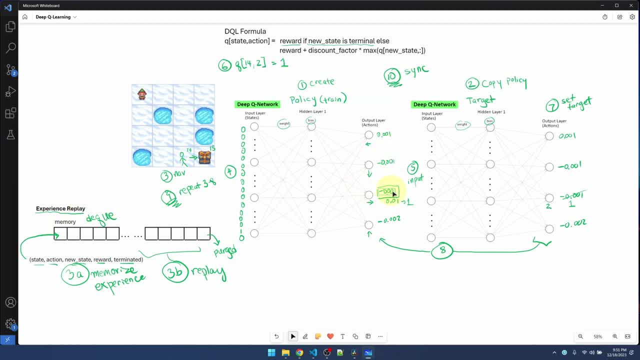 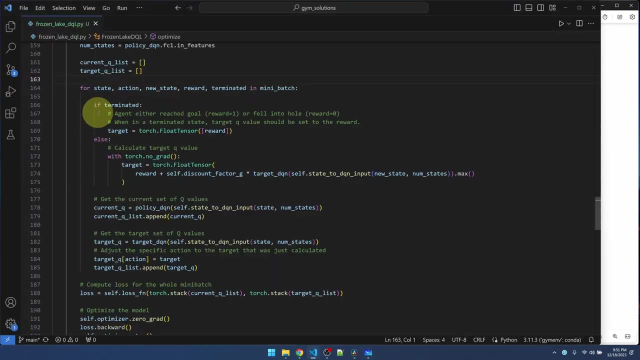 which should be the same as the queue values from the policy network. Step number 6 is up here, So a reminder of what it looks like. Step 6 is using this formula here, So that's what we have here, If terminated. 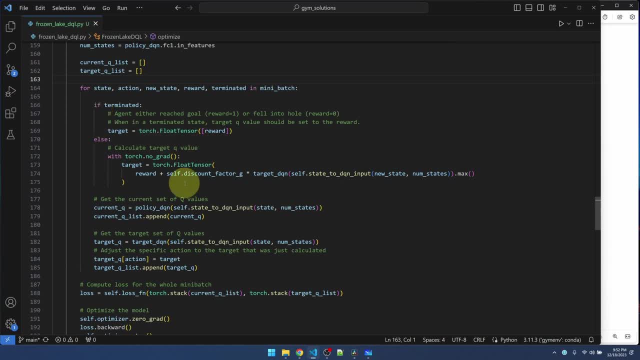 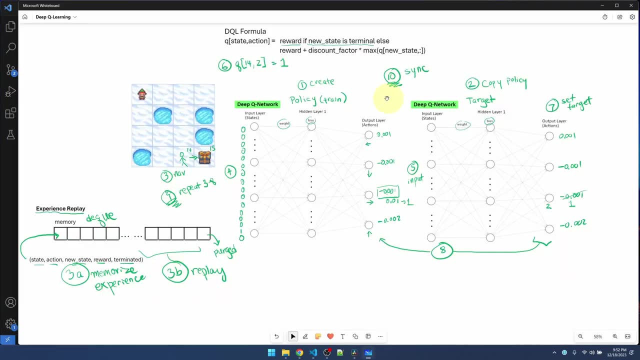 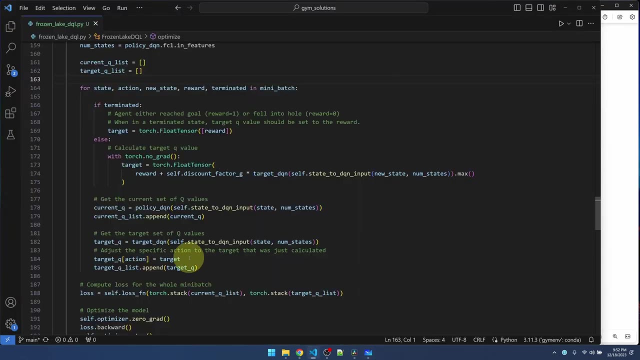 If terminated, just return the reward. Otherwise, use that second formula. So now that we have a target, we'll go to step 7.. Step 7 is taking the output of step 6 and replacing the respective queue value, And that's what we're doing here. 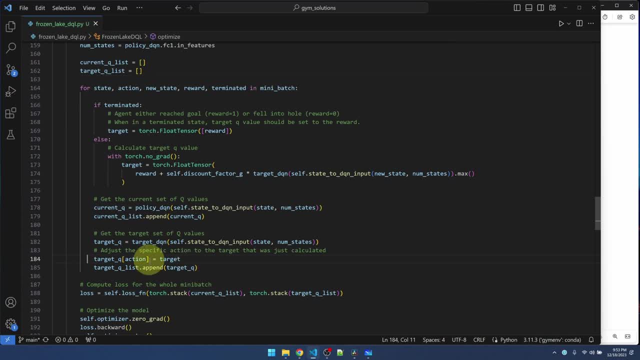 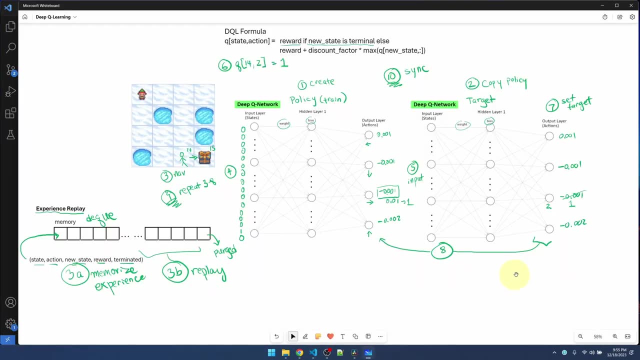 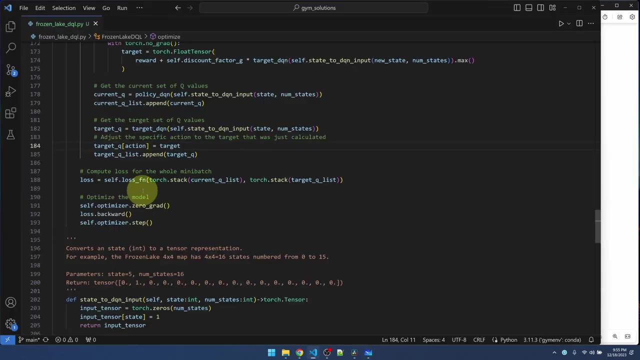 We're replacing the queue value of that particular action with the target that was calculated up above Step number 8.. Step 8 is to take the target values and use that to train the current queue values. So that's what we have here. 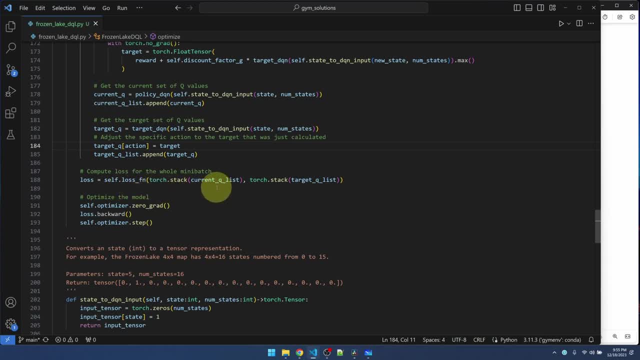 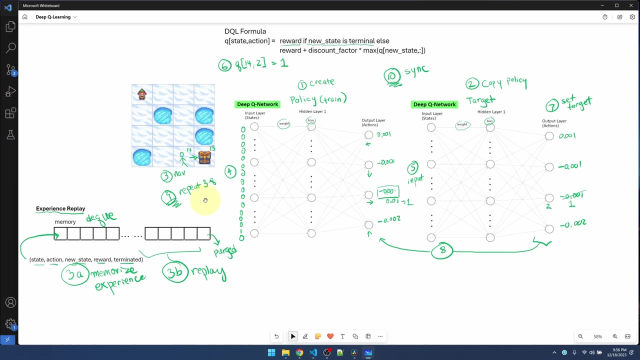 We're using the loss function Pass in the current set of queue values plus the target set of queue values, And then this is just standard PyTorch code to optimize the policy network. Now step 9.. Step 9 is to repeat steps 3 to 8,. 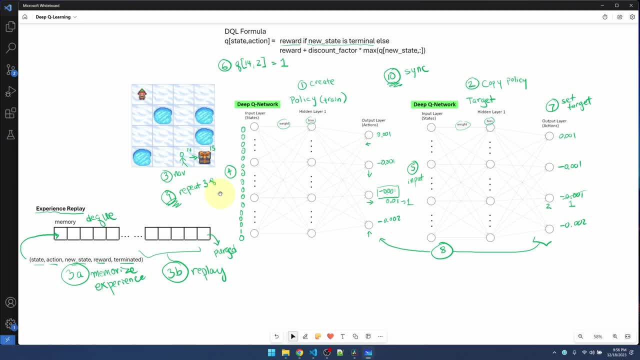 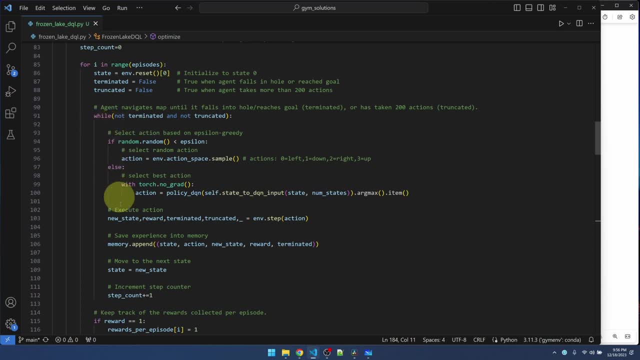 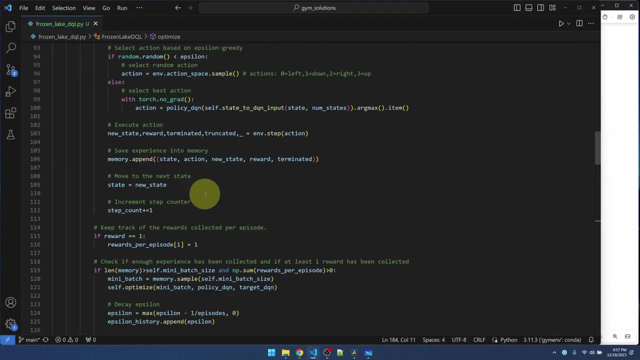 starting from navigation to optimizing the network. Basically, that's just continuing this inner while loop of stepping through the states and this outer for loop of stepping through each episode. Step 10 is where we sync the policy network and the target network And we do that down here. 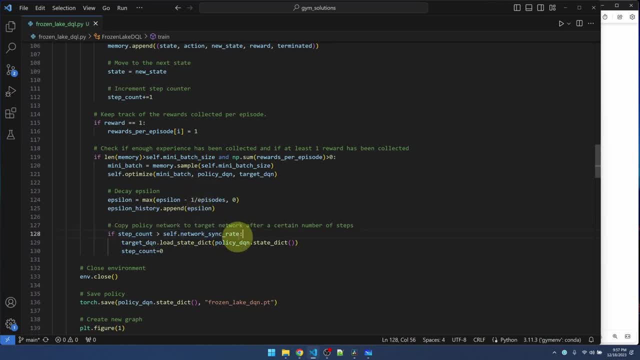 If the number of steps taken is greater than the network sync rate that we set, then we copy the policy network into the target network And then we reset the step counter. Also, after each episode we should be decaying the epsilon value. 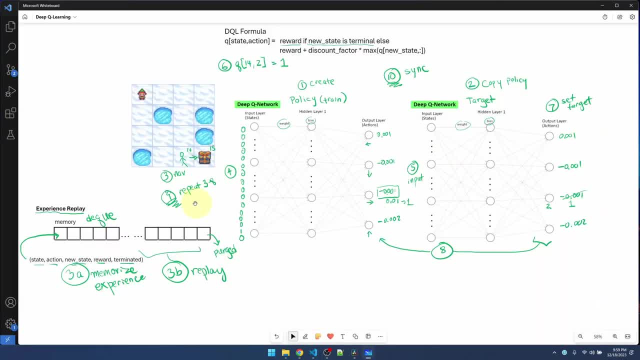 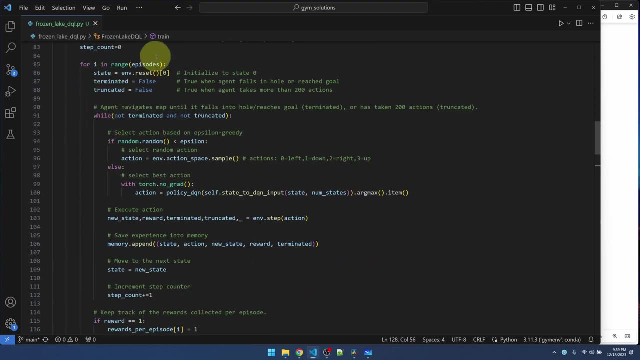 After syncing the network, we repeat step 9 again, which is repeating basically the navigation and training again. So it's just going to go back up here and do this all over again all the way until we have finished the number of episodes. 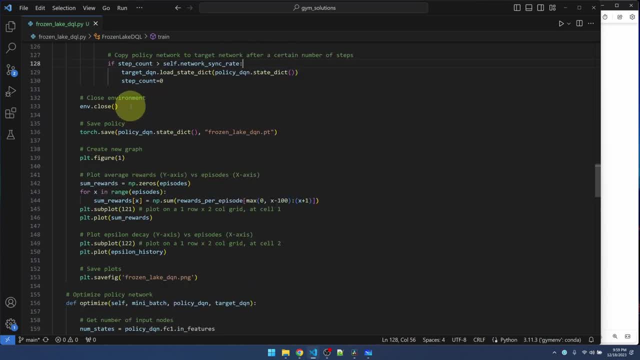 So that was training. After training, we close the environment. We can save the policy or the weights and bias into a file. I'm hard coding it here. You can definitely make this more dynamic. Here I'm creating a new graph. 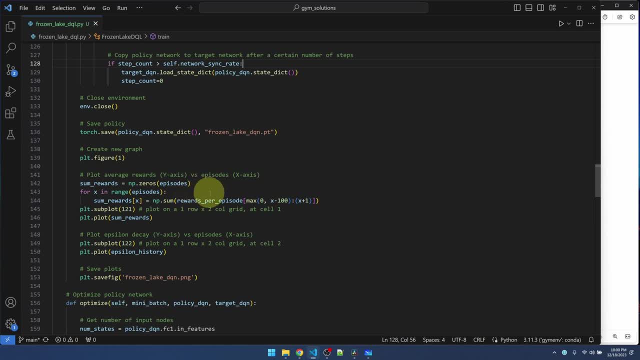 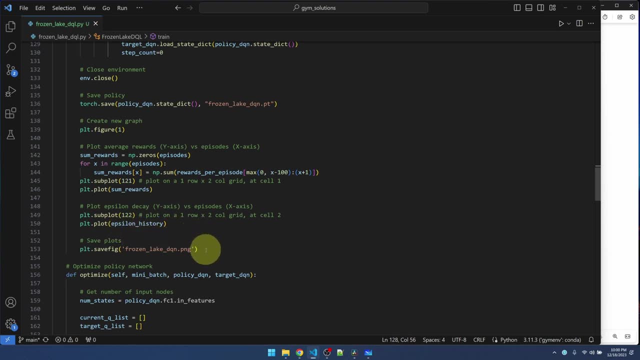 And I'm basically graphing the rewards collected per episode. Also, I'm graphing the epsilon history here. After graphing, I'm saving the graphs into an image. All right, So that was the train function. We already talked about the optimize function. 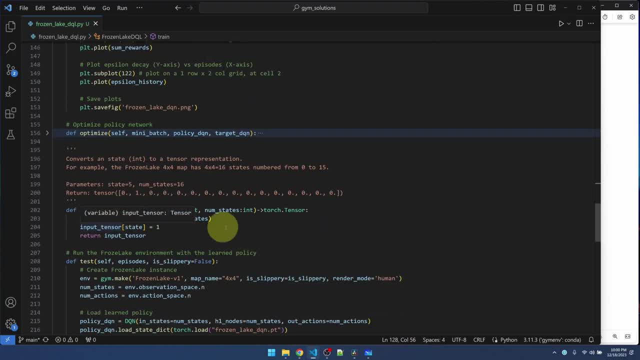 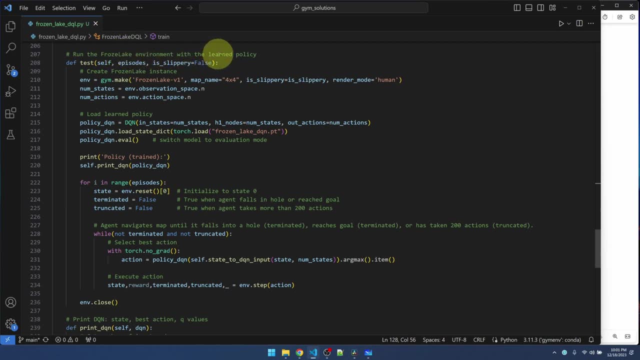 Let me fold that. We already looked at that. Now the test function is going to run the frozen lake environment with the policy that we learned from the train function. We can also pass in a number of episodes and whether we want to turn on slippery or not. 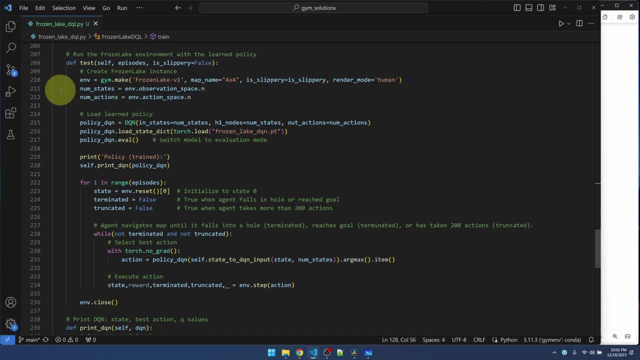 So the rest of the code is going to look pretty similar to what we had in the train function. We instantiate the environment, get the number of states and actions 16 and 4.. Here we declare the policy network load from the file that we saved from training. 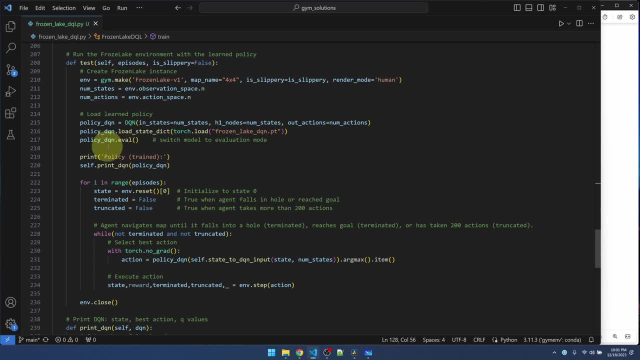 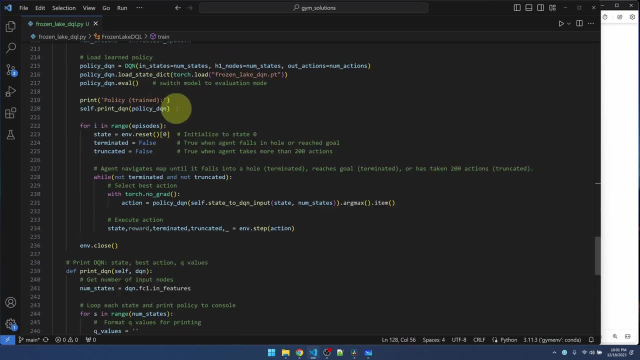 This is just PyTorch code to switch the policy network to prediction mode or evaluation mode rather than training mode. We'll print the trained policy and then we'll loop over the episodes. We set the agent up top. You've seen this before. 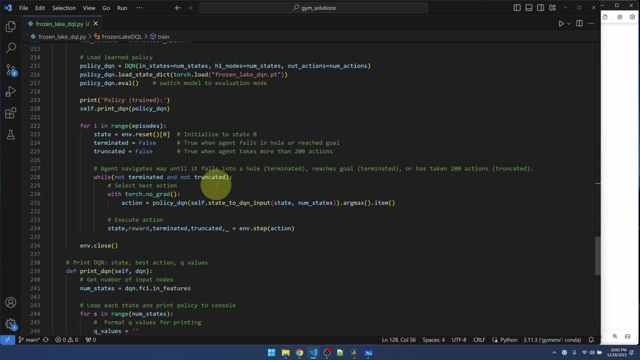 Keep looping until the agent gets terminated or truncated. Here we're selecting the best action out of the policy network and executing the action and then close the environment. So ideally, when we run this, we're going to see the agent navigate the map. 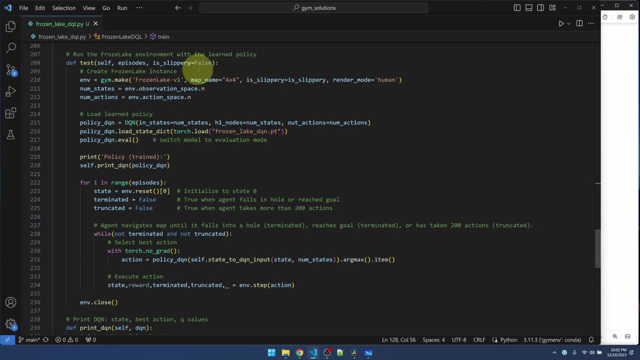 and reach the goal. However, if slippery is on, there is no guarantee that the agent is going to solve it in one try. It might take a couple of tries for the agent to solve the map All right down at the main function. 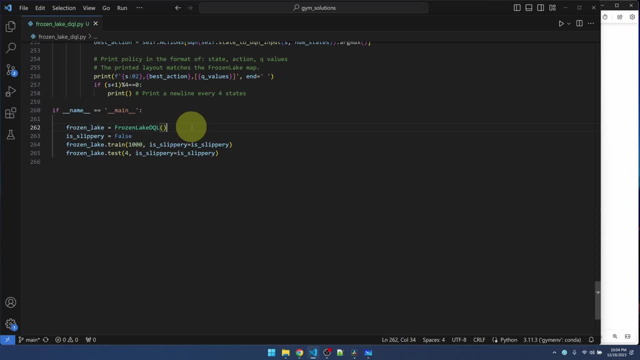 we create an instance of the Frozen Lake DQL class First. we're going to try non-slippery. We'll train it for a thousand times or a thousand episodes. We'll run the test four times just because the map pops up and goes away. 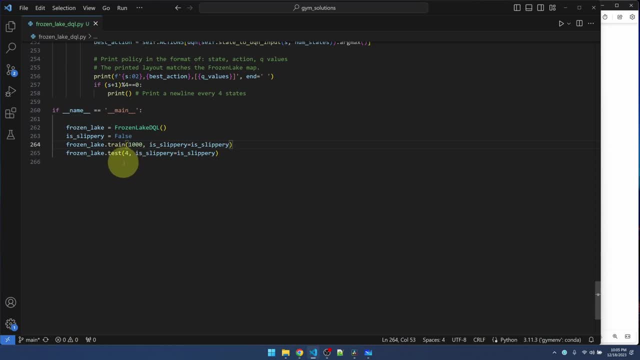 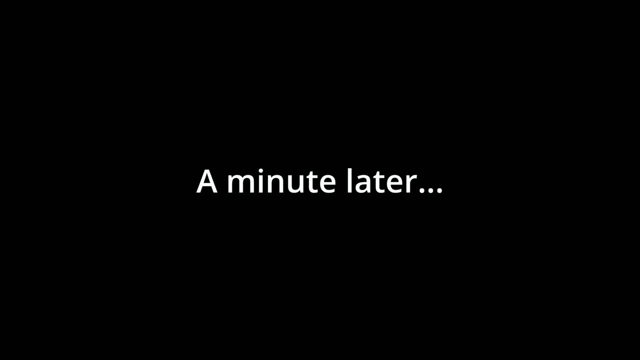 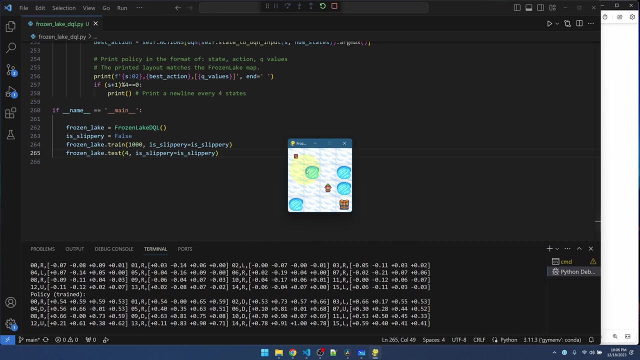 when the agent gets to the goal. So we want to run it a couple of times so we actually can see it on the screen. Okay, I'm just hitting control F5.. All right, training is done and it looks like the agent is able to solve the map. 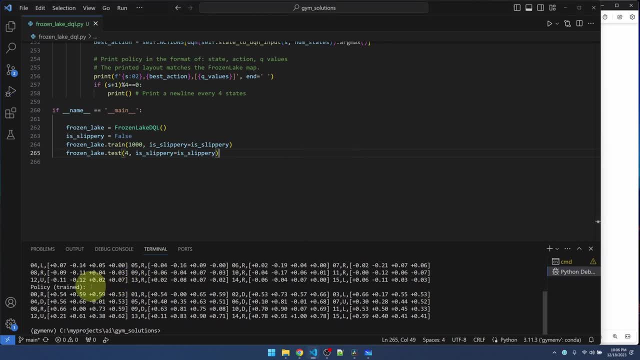 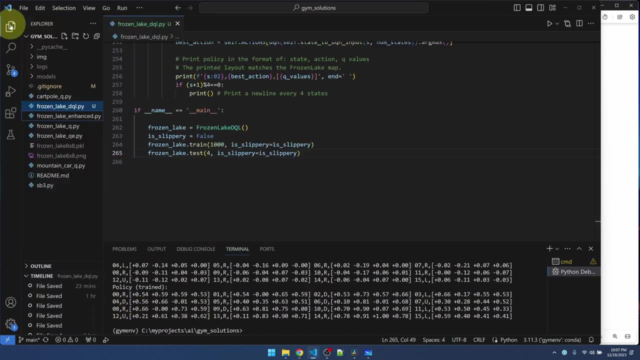 We also have a printout of the policy that it's learned. I print it in a way that matches up with the grid. Let's jump back to this in a second. Let's go to our files. So, after training, we have a new graph. 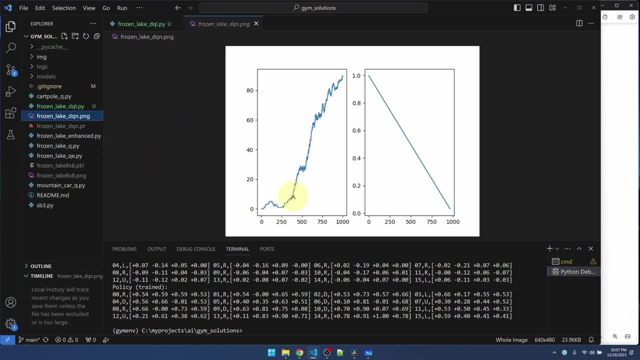 On the left side, that's the number of rewards collected over the 1,000 episodes. As you can see, over time it's improving and finally, at the end, it's getting a lot of rewards. On the right side, we can see epsilon decaying. 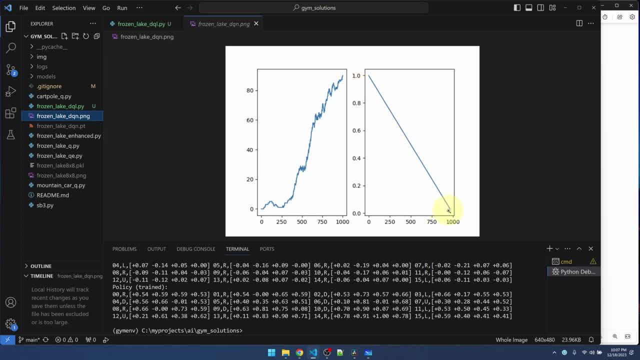 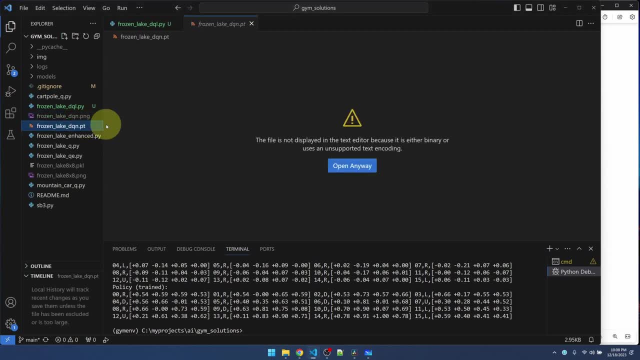 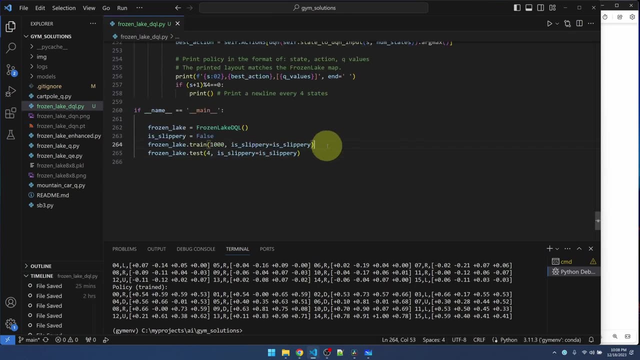 starting from one, slowly, slowly down to zero. Also, another file that gets created is it's a binary file, so we can't really display it, but it contains the weights and biases of the policy network. So if we want to do the test again, 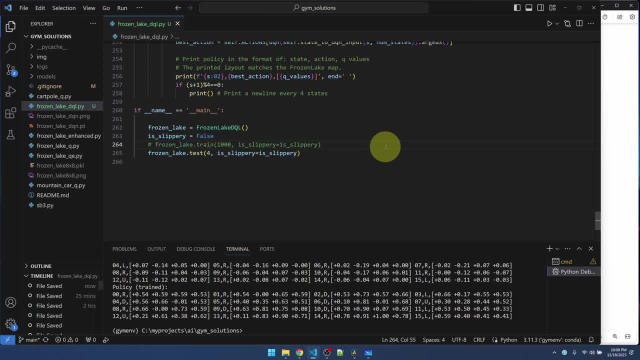 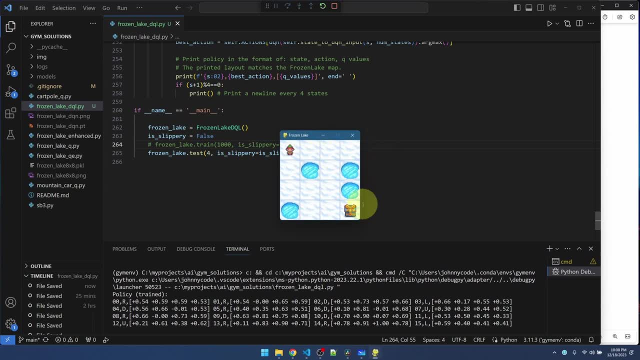 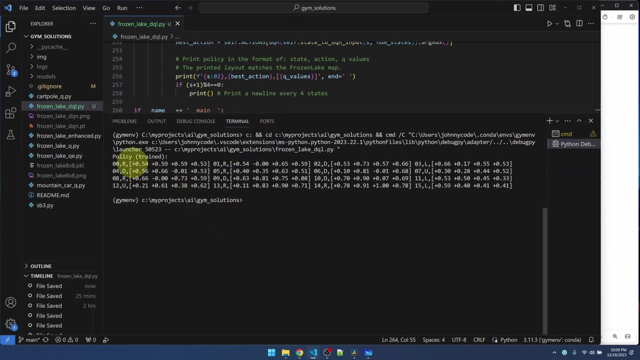 we don't need the training. We can comment out the training line and just run this again and we can see the agent solve the map. We can look at what policy the agent learned, The way this is printed. it matches up with the map. 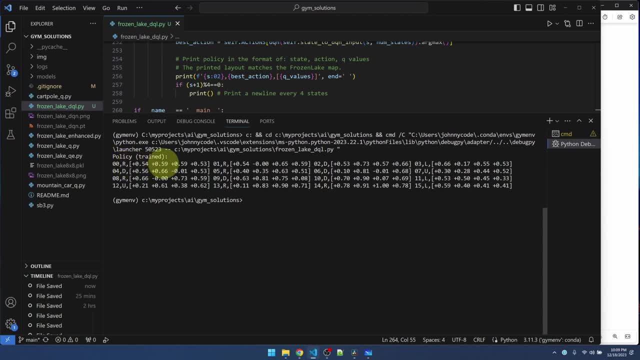 So at state zero, the best action was to go right, which is state one. At state one, the best action is to go right again. At state two, go down. At state six, go down again. At state ten, go down again. 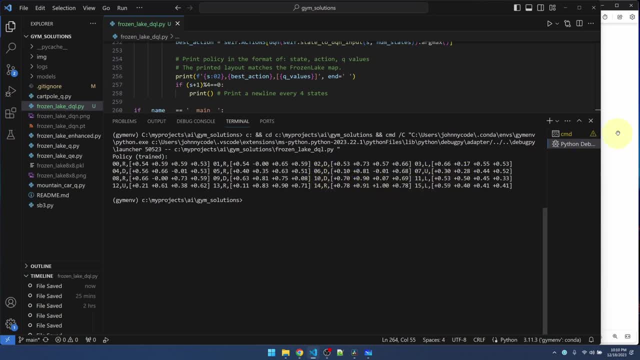 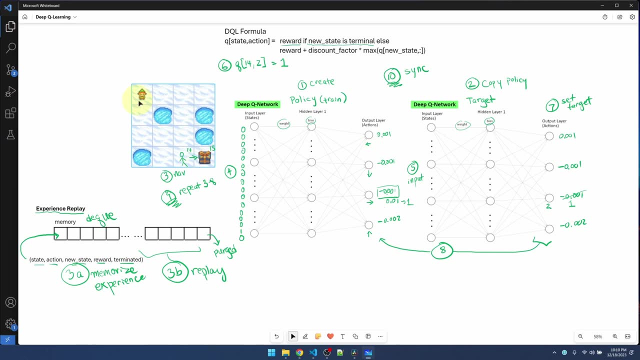 At state fourteen go to the right. Okay, So it was right right down, down down right. So remember earlier that there were two possible paths: the one that we actually learned plus the one going down, Because epsilon greedy has a randomness factor. 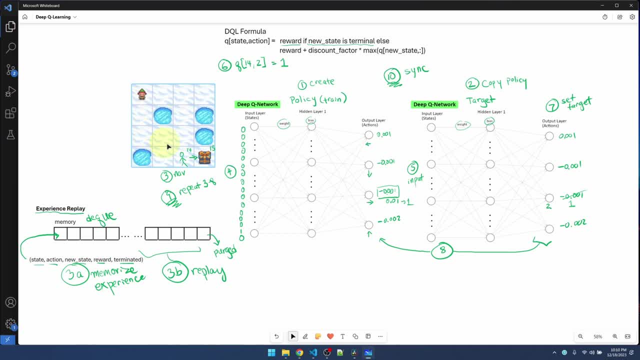 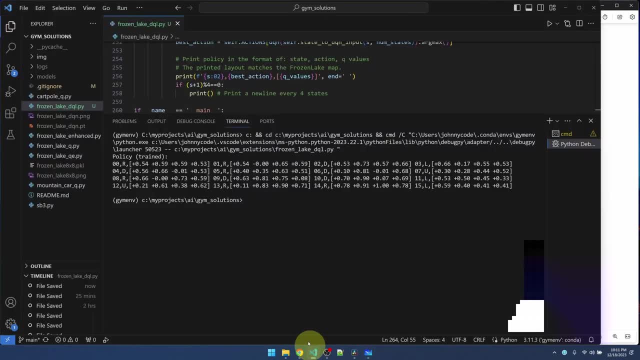 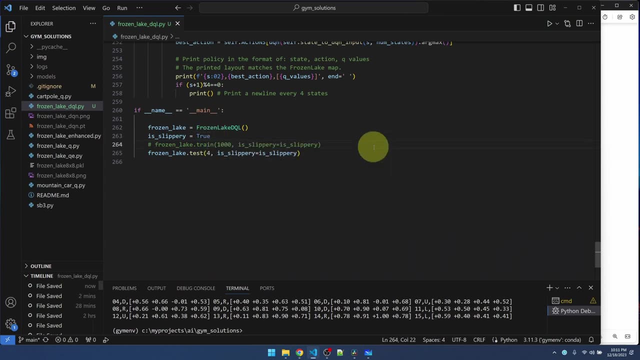 whether the agent learns the top path or the bottom path. it's just somewhat random. If we train again, maybe it'll go down the next time. Now let's turn the slippery factor on. Uncomment the training line Now with slippery on. 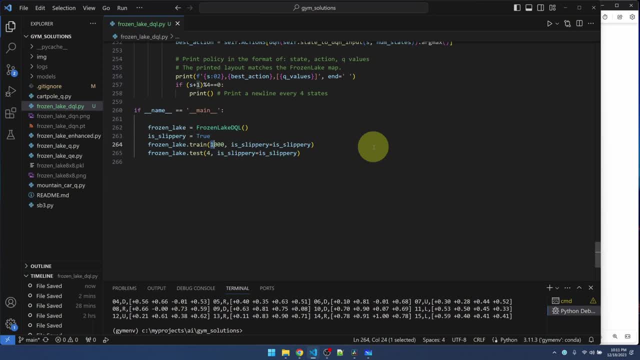 we expect the agent to fail a lot more often or to fall in the holes a lot more often. Let me just triple the number of training and let me do it ten times for testing. Okay, I'm running this again, Again, with slippery turned on. 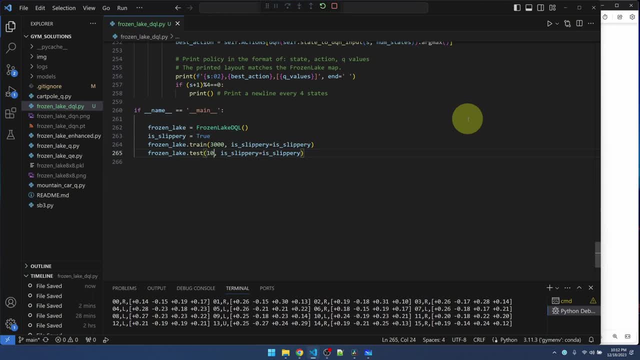 there's no guarantee that after training, the agent is going to be able to pass every episode. Let's make it come up. You see it trying to go to the bottom right, but because of slippery it just failed right there. But there you go. 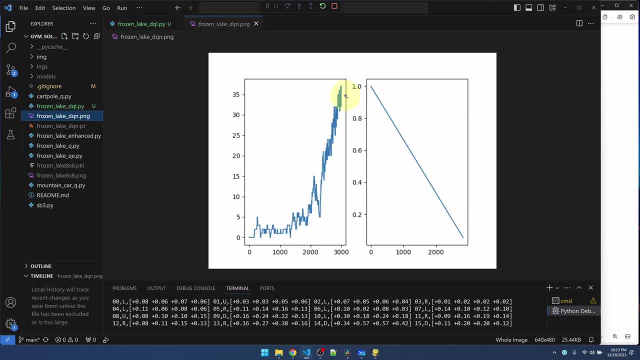 It was able to solve it. Now let's look at the graph. The results compared to the non-slippery surface is significantly worse. Also, you want to be careful getting stuck in spots like these, which means if I was unlucky enough to set my training episodes to maybe 2200.